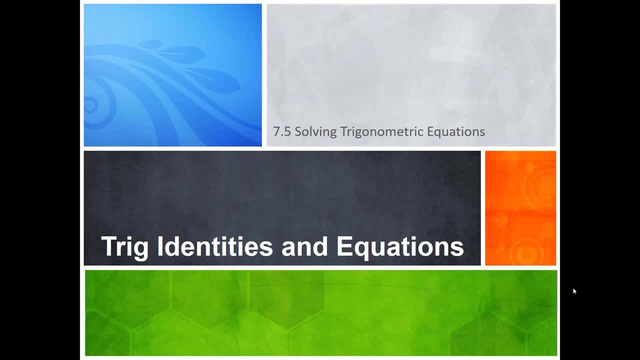 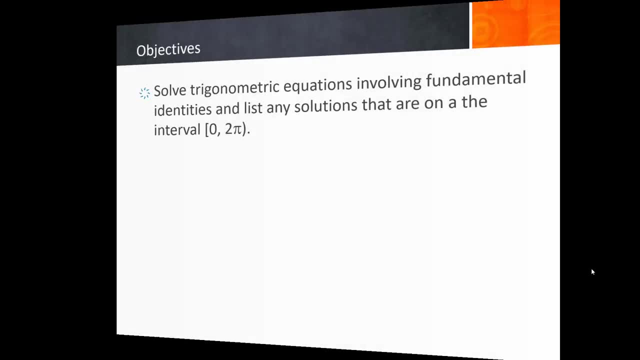 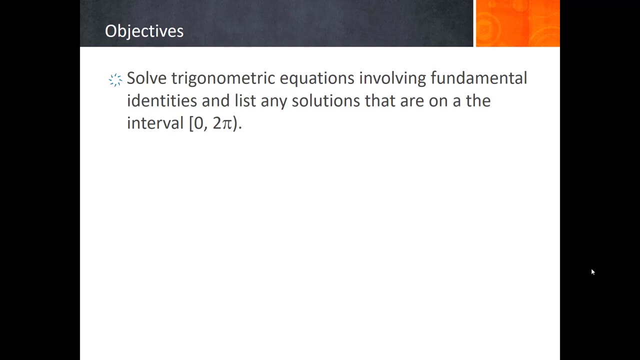 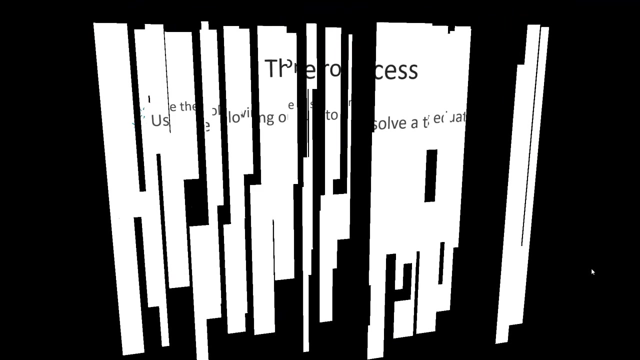 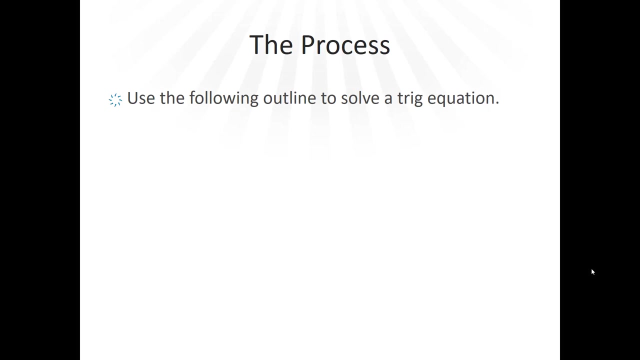 Welcome to a video on solving trigonometric equations. In this lesson we'll look at just solving basic equations using just kind of some simple algebraic techniques and then we'll come back in another video in a few weeks and look at how we can incorporate all those identities that we just learned about how do we use them to also solve equations. But for now we just want to kind of look at what does it mean to solve an equation and again just some of the basic ideas. When we solve an equation there are two ways that we can express the solution. One is we can express just all the answers and there could be more than one, there generally will be more than one, but all the answers between zero and two pi. So if you remember zero to two pi is going to represent one complete loop, one complete cycle around. The unit circle and then we also have a technique that we use to express the fact that there are actually infinitely many solutions because you can keep going around the unit circle forever in both the positive or the negative direction. So let's look at the overall process that we can follow to solve trig equations and again we won't look necessarily at all these points but we'll look kind of at most of them in this video. So the first step that you would want to do is to simplify your equation. 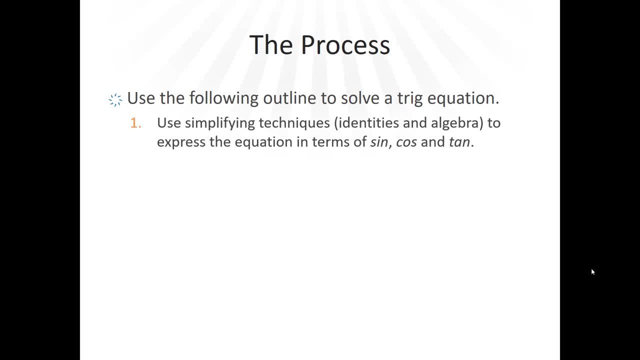 Now for again right now that's primarily just going to be an algebraic process. 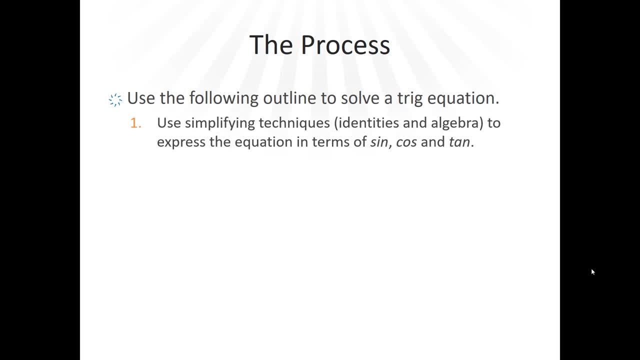 We are going to look at specifically you know just some simple arithmetic adding and subtracting numbers back and forth dividing numbers or factoring maybe some square roots stuff like that. 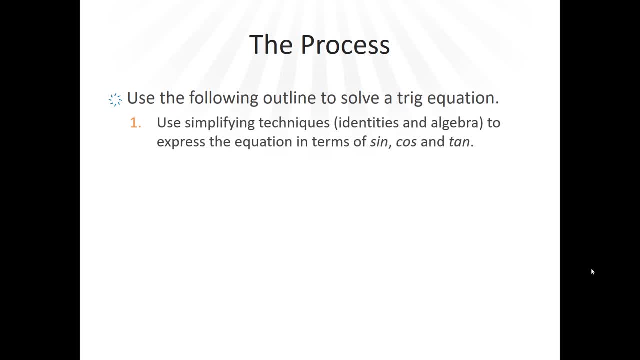 And then in a few weeks we'll come back and we'll look at how do we take the identities that just learned and combine that into this process but for now it's just going to 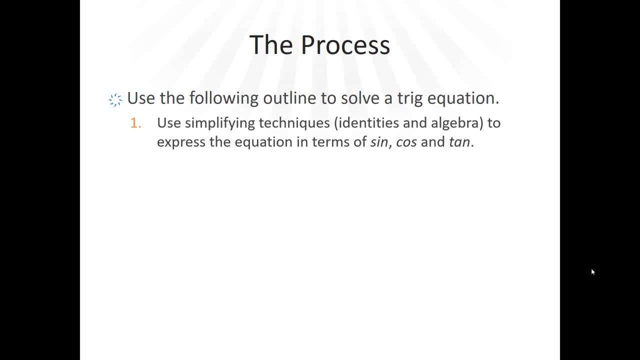 be kind of basic algebraic stuff and we're just going to simplify it when you have the identities you want to make sure you have the equations all written in terms of sine cosine and tangent it's like you have those reciprocal 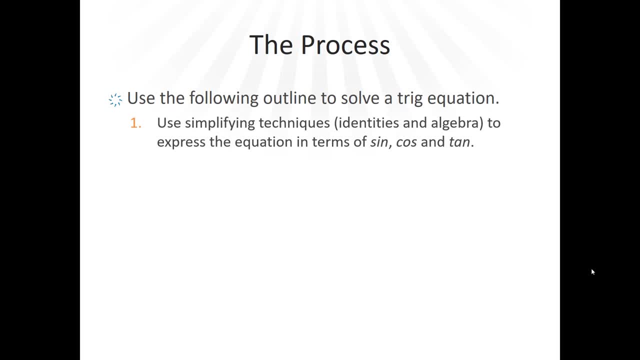 identities that would let you convert you know cosecant to sine so once we have our simplified equations and we have them all in terms of sines cosines or tangents we want to determine the solution for the sine cosine and tangent 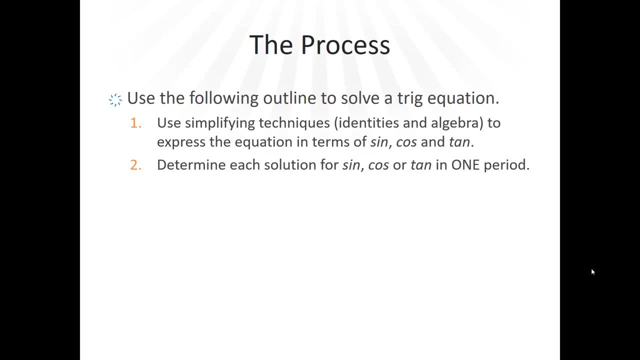 equations in one period okay now when we think about the period length for sine and cosine remember that's a length a period length of 2 pi if you remember back to our graphs and again that represents a full loop around the unit circle tangents a little different tangent has a period length of only pi and so when we talk about the answers in one period we really only have to find the answers depending on the textbook you may you read it may say is finding the answers from negative pi over 2 to positive pi over 2 because that's usually kind of the standard period or you could talk and that's the way we'll do it we're going to talk about how do you find the answers just between 0 and pi that way we keep our values all positive so usually for sine and cosine we're looking between 0 and 2 pi for tangent in the larger scope you only need to look at answers between 0 and 1 pi but ultimately we're going to want answers everywhere so once we can kind of find those answers we want to look at how we can express all the solutions okay and so we do that by adding this sort of we call it an 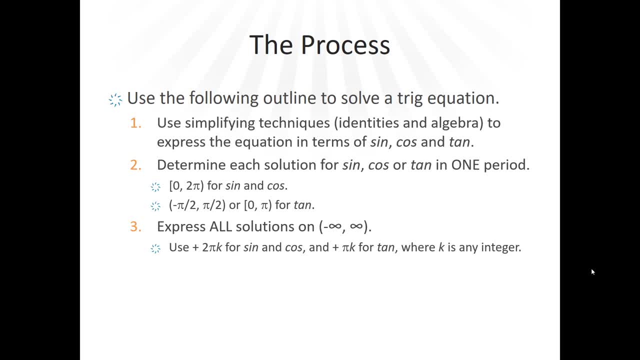 arbitrary constant in this case we use the letter K some text may use the letter N or a different letter but K just represents an integer so if you remember integers are all the positive and negative whole numbers so 1 2 3 4 5 0 and negative 1 negative 2 negative 3 and so forth so what we do is again remember that sine and cosine have a period of 2 pi so that means going once around the circle if you keep going another time you're going to have a period of 2 pi so that means going once around the circle if you keep going another time around the circle and another time around the circle you'll keep ending up at the same spot on the circle when we have those coterminal angles and so for sine and cosine we're going to add to our answer we're going to add a little expression we're going to do plus 2 pi K okay so that plus 2 pi K just shows us that there are in addition to the one specific answer we list there are infinitely many coterminal answers to that I'm going to show you how to do that in just a second I'm going to show you how to do that in just a second 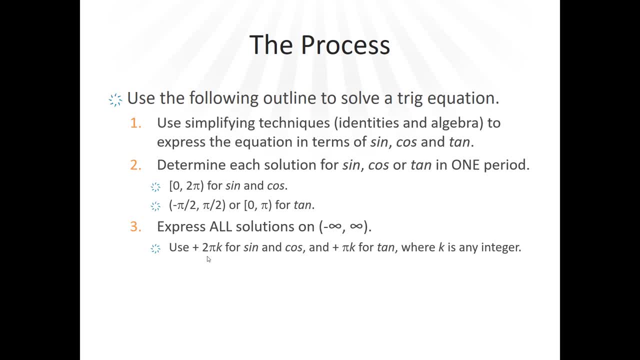 which is going one more time or two more times or three more times around the circle in either the positive or negative direction again that's because 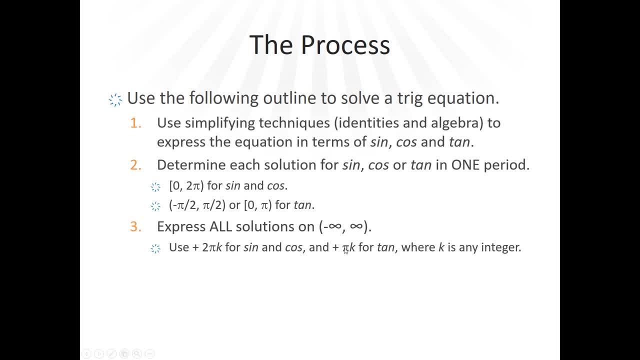 of K's in integer and then for tangent again tangent is has a period of just 1 pi so instead of adding 2 pi to the answer we'll add just a pi K alright and 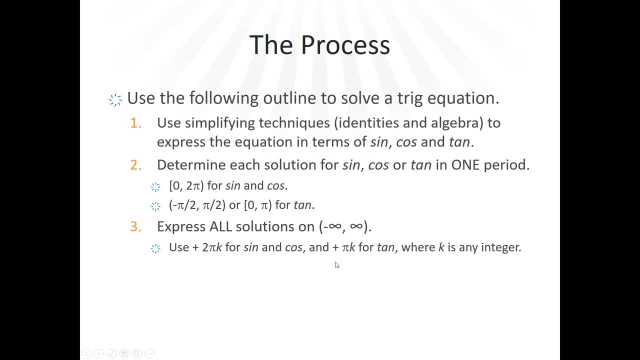 so we'll see what that looks like in practice here in a few examples and in addition to listing all solutions we want to be able to list any specific solutions that are on the interval from 0 to 2 pi so within one cycle of the unit 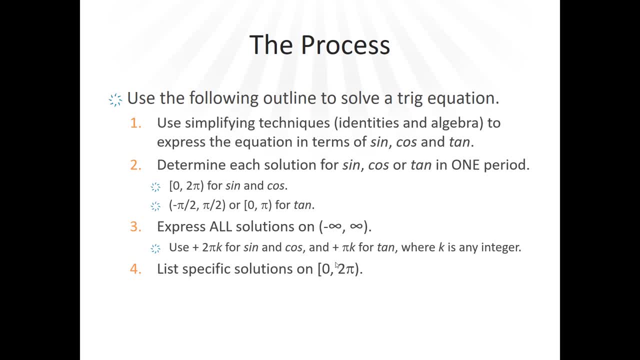 circle what are all the answers and sometimes we made kind of steps 3 and 4 we may flip around a little bit and kind of merging with step 2 a little bit so it's not necessarily like real extinct steps here that we're kind of doing each one separate from the other it's just you can kind of enter enter play some of these steps with each other a little bit 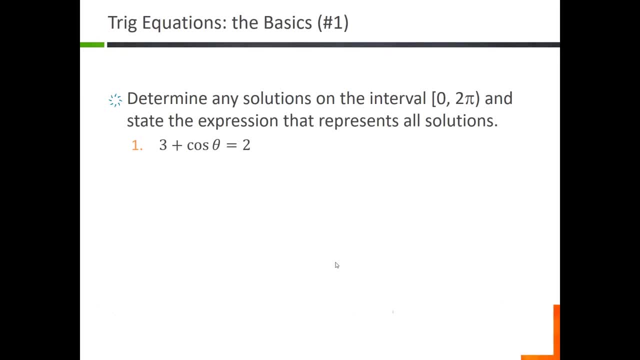 so let's just work through a bunch of examples here we'll start out again fairly easy just doing some basic algebra and then we'll look at some examples that involve maybe square root and then some factoring okay so for this 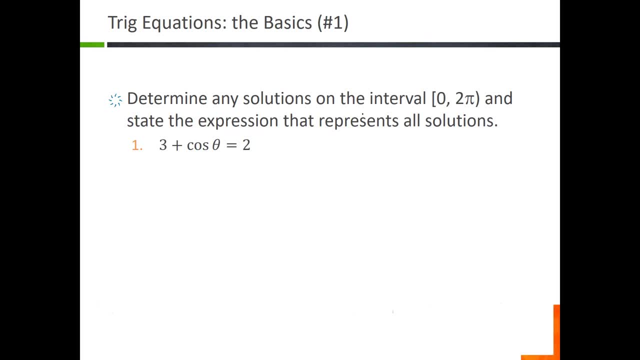 first example we want to determine any solutions on the interval from 0 to 2 pi so remember that was one of those the last step in that process but we can again change that order around a little bit but we want to find any solutions on the interval from 0 to 2 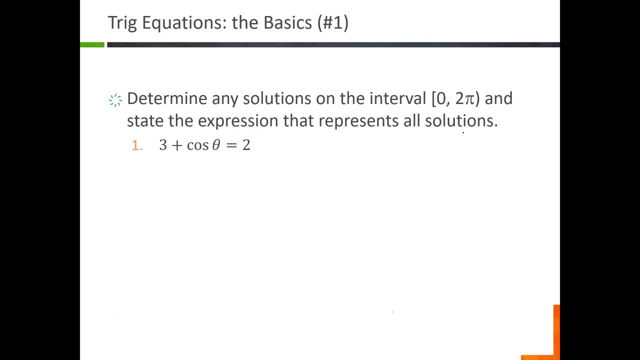 and we want to state the expression that represents the all answers, the infinitely many solutions. Okay for this first example we have 3 plus cosine of theta is equal to 2. So in order to solve the equation again remember our first step was to simplify the equation and so when we want to simplify it if you just think about solving a normal equation so say just you know go back to like an algebra class if you had 3 plus x was equal to 2 in order to solve it you would isolate your x right so you'd subtract 3 from both sides which the 3s on the left side cancel out and you're left with x is equal to a negative 1. So we're in essence doing the same thing we're going to solve it in terms of cosine of theta first. So we have 3 plus cosine of theta is equal to 2. 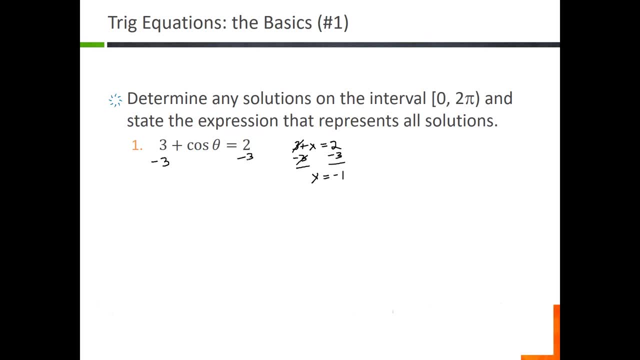 We're still just like we would in algebra we're going to subtract 3 from both sides which that leaves us with the cosine of theta is equal to a negative 1 just like it did before in algebra. So this is where the trig comes into play. We want to find any values for theta that makes cosine of theta equal to a negative 1 and to do that again we want to think about 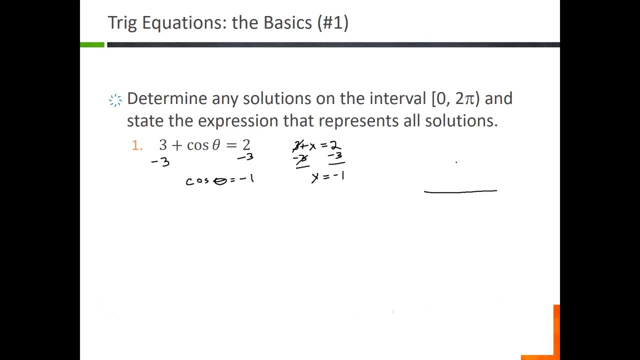 our unit circle. So let's go ahead and just draw it out and we're going to do that. So let's go ahead and just draw it out and we're going to draw it out and we're going to do that. So let's go ahead and just draw it out and we're going to draw it out and make a rough sketch of our unit circle. 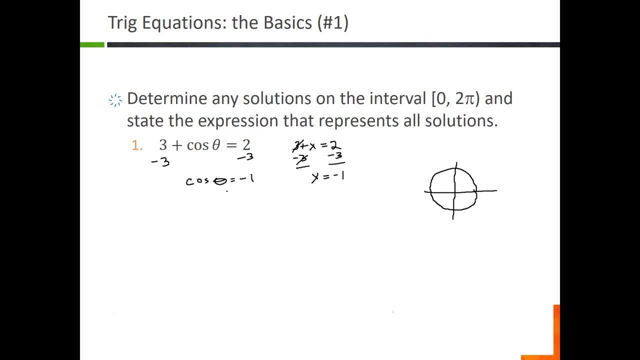 Okay so we want to know when cosine is a negative 1. So remember cosine is the x-coordinate so we want to know which points on the unit circle have an x-coordinate of negative 1. It turns out that that is one of the quadrantal angles it's on the negative x-axis and that is an angle of 0 or sorry not 0 but 100. So we want to know when cosine is a negative 1. So we want to know when cosine is a 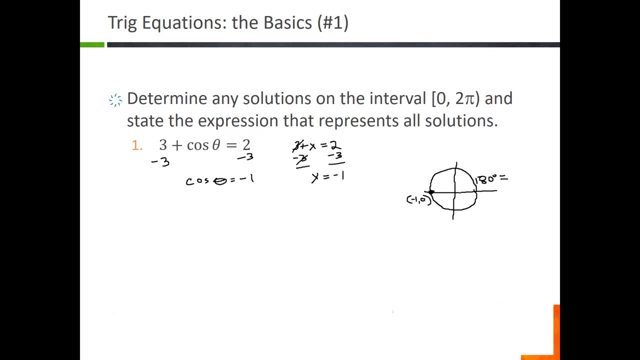 So let's go ahead and draw out the rokuatching equation for tane. So the ありant angle is the Karma Single pueden be written as a Dit 1978, tornado, emergency earthquake,事情 der 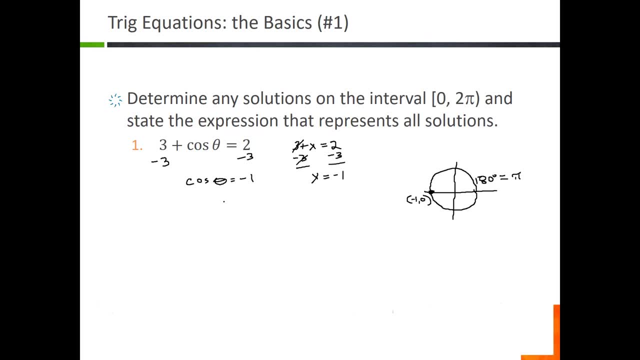 mess in the city etc and the problem with the Saturn area of Saturn is that it runs at a velocity of 180 degrees but we don't want to deal with degrees since we want to look for the answer between 0 and 2 pi. We want to think of this in terms of radiance. So pretty much all of our work in here is going to be in radiance. So pretty much all of our work in here is going to be in radiance. The angle to the negative x-axis is going to be pi radians. okay so that's the only angle between 0 and 2 pi the only number between 0 and 2 pi that will make cosine equal to 1 so theta is equal to pi this is the answer 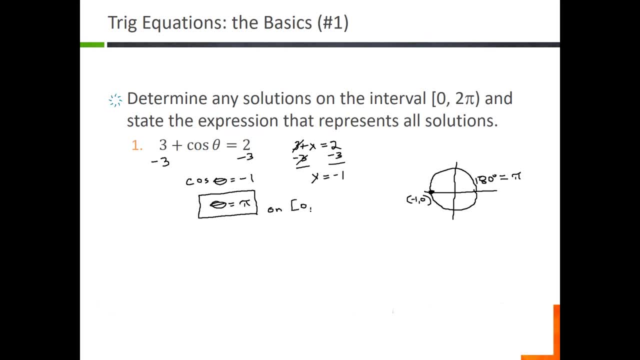 that we have on the interval from 0 to 2 pi okay so that's the first part of our problems we want to figure out that solution the second part is we want to state the expression that represents all solutions so if you remember on the previous slide there we talked about how we could add an additional expression and for sine and cosine we're going to do plus 2 pi K so what our answer would look like and it's really easy we're just going to put that 2 pi K on the ends we're going to have the original pi plus a 2 pi K 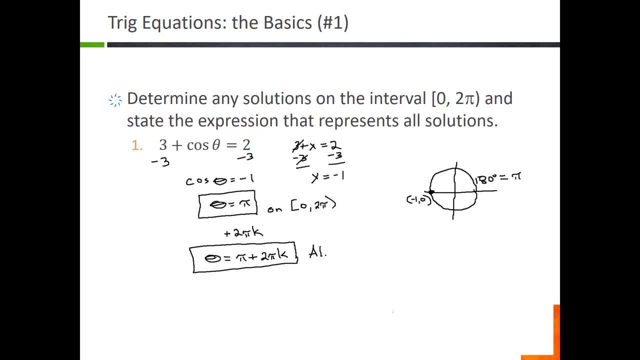 okay and this is the answer for all solutions so what is exactly does that mean let's go back to our unit circle here so according to our first answer we 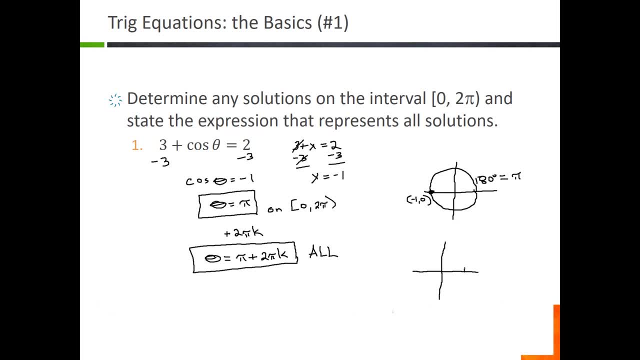 know that if we were to rotate along the unit circle for pi radians we would end up with a point on the unit circle and that'sadax that point on the unit circle has a coordinate of negative one zero and cosine of pi then has to be a negative one so that satisfies the original equation that we have but what happens if we continue to rotate how far do we have to rotate to end up at the same place so if we take if we start that rotation of pi and then say we rotate another distance of two pi well it turns out that I end up at the same point and what if I were rotating again another distance of two pi well I'd end up at the same point and if I rotated again a distance of two pi I'd end up in the same point what if I rotated in the other direction a distance of two pi well I'd end up with the same point but now it's a negative two pi and so anytime I rotate an additional two pi whether in the clockwise or counterclockwise direction I will still end up at the same point and so that means any point that has pi plus a multiple of two pi I will always end up here on the negative x-axis at negative one zero and those are all points that you 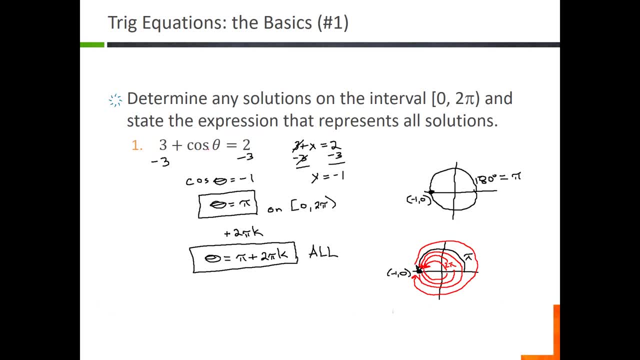 make cosine equal to a negative one which makes three plus cosine equal to a two so and there's infinitely many times that I can rotate around this and so that's why we can't obviously express an infinite number of answers by listing them out so we need an expression that summarizes that and that's what this plus two pi k is okay it gives us a summary 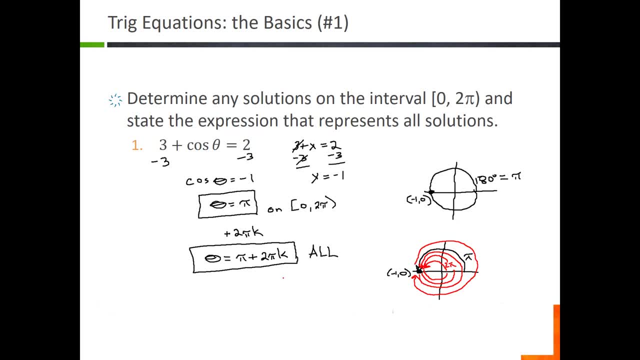 of all of those infinitely many answers 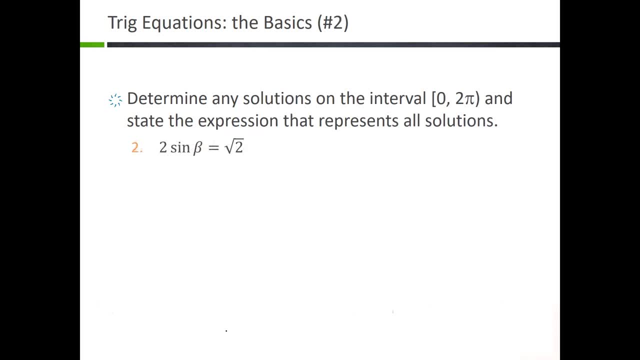 all right let's look at another example so we have two times the sine of beta is equal to the square root of two and again we want to find all the solutions between zero and two pi and then we want to state all solutions for the infinitely many rotations around the circle 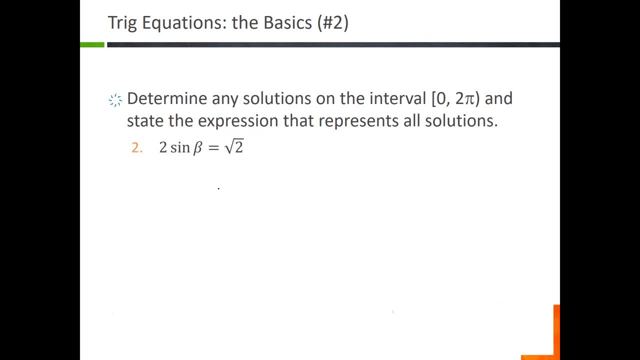 so again our first step is to simplify and again we're just doing basic algebra here so we could go ahead and divide both sides by two and so that's going to give us the sine of beta of beta 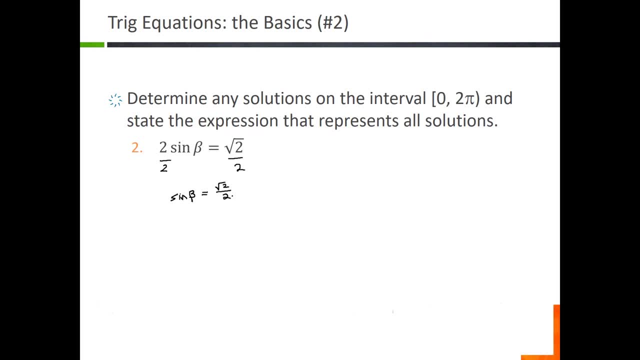 Is equal to a square root of 2 over 2 so once we've simplified it We pretty much have to go back to our unit circle every time. That's the whole point of this 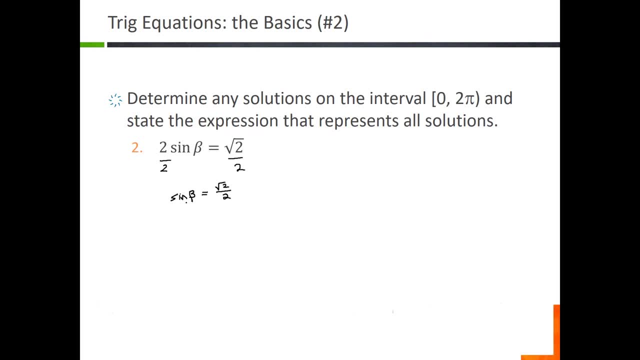 Is to simplify it down to a nice simple expression? involving sines cosines and tangents 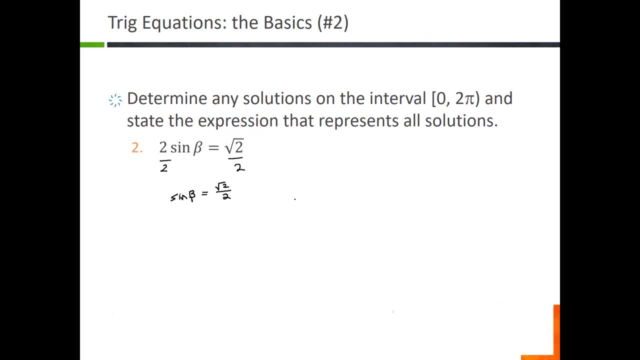 Hopefully it's a number on the unit circle Which we can find the exact solution if not we may have to use our calculator, so let's think about where sine is 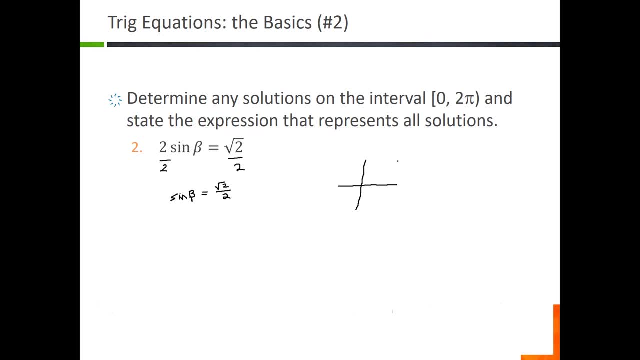 equal to a root 2 over 2 so we know sine is positive in the first and the second quadrant, and this is a positive root 2 over 2 not a negative root 2 over 2 and 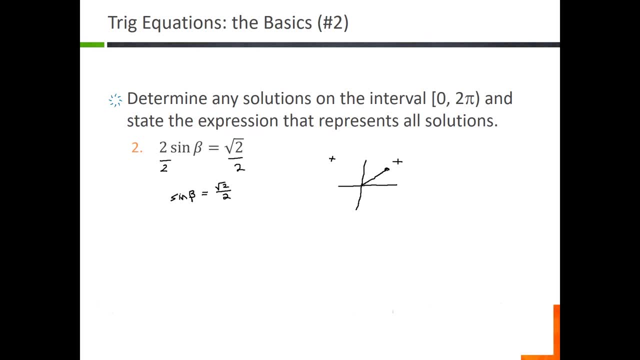 So we know That sine is a positive root 2 over 2 at two locations 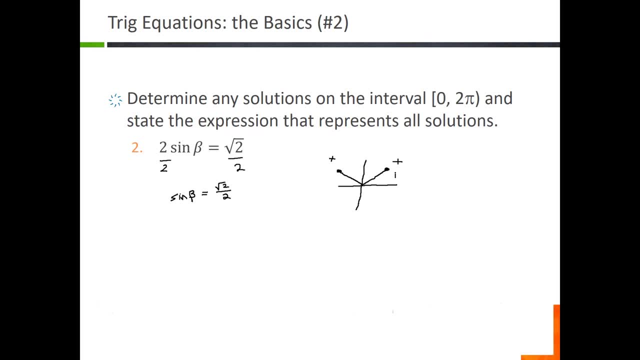 It will be a root 2 over 2 when beta is a pi over 4 radians or when it is 3 pi Over 4 radians and so those are the two answers that we are going to get so we get beta is equal to pi over 4 comma 3 pi over 4 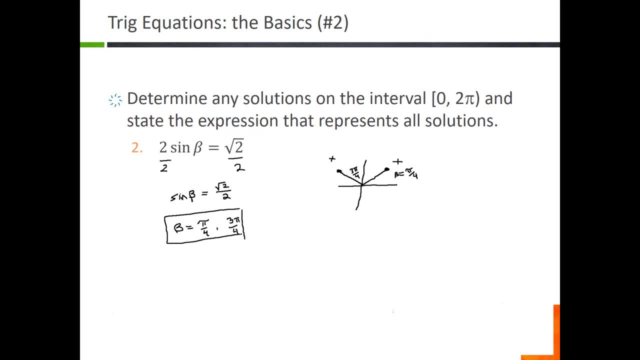 And again, those are the answers those are the only answers between 0 and 2 pi 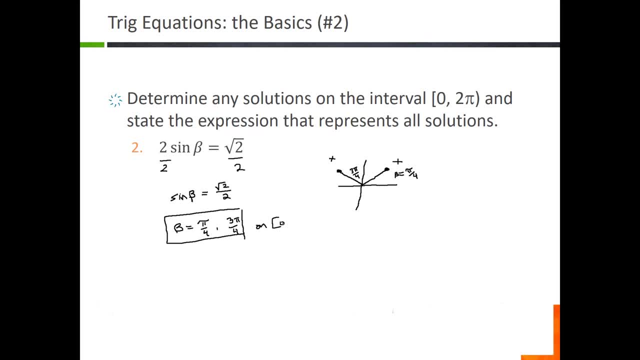 Okay, so those are the answers on the interval from 0 to 2 Pi 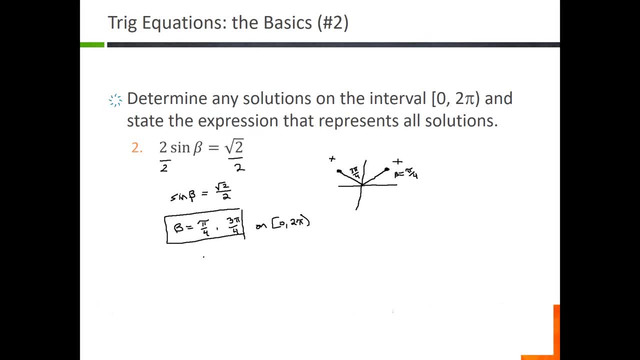 So how do we express the fact that there are infinitely many answers? So again, we're going to take each of these and we're going to add in that little extra Expression so we have beta is equal to pi over 4 plus 2 pi K and We're going to have a second expression. We're going to have beta is equal to 3 pi over 4 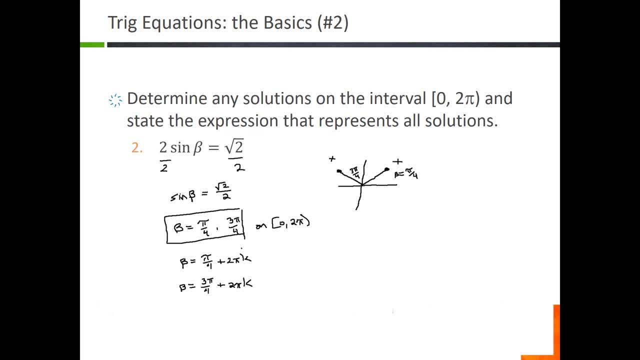 plus 2 pi K and in order to express all Of the solutions we have to have both of these expressions Okay, if you didn't write the second one If you only wrote the pi over 4 plus 2 pi K You would only get the angles that are co-terminal in the first quadrant And if you didn't do the pi over 4 but instead wrote 3 pi over 4 plus 2 pi K You would get the infinitely many answers that are co-terminal in the second quadrant, but we have both of these that we have to include so make sure that we have 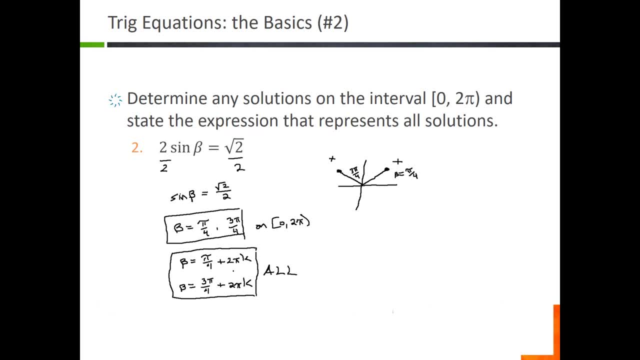 Now we may eventually see some problems where it is possible to combine these sort of merge them into just a single expression But neither of these examples we've looked at so far would allow us to do that 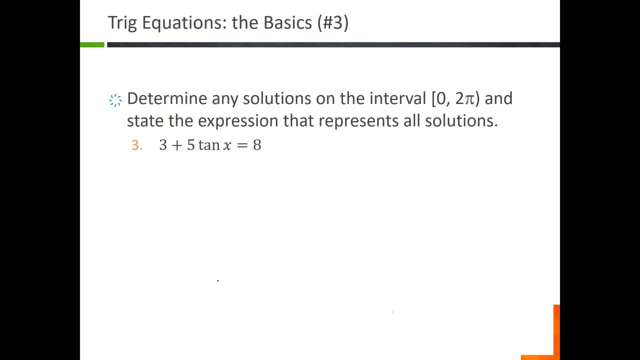 Alright, let's look at a third example this time involving tangent so we have 3 Plus 5 times the tangent of X is equal to 8 so again our first step is just basic simple algebra right now We'll get into more complicated stuff later 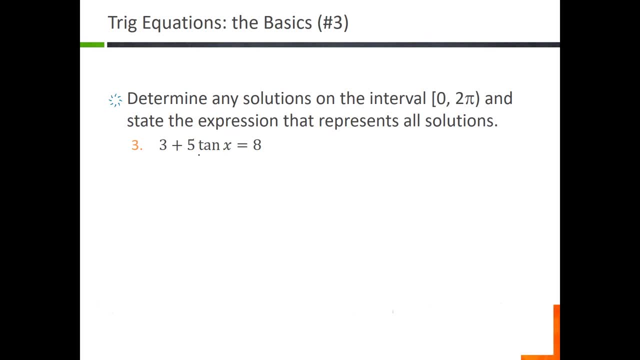 But again just treat this like a normal algebraic expression if we're trying to solve for X we need to isolate it Which means we need to move stuff around back and forth so the first step We're going to do is subtract 3 from both sides of the equation And that leaves us with 5 times the tangent of X Is equal to 5 and then we're going to divide 5 into both sides of the equation and that's going to give us the tangent? Of X is equal to 1 So we just two steps of algebra, and we got it simplified down to a nice and easy 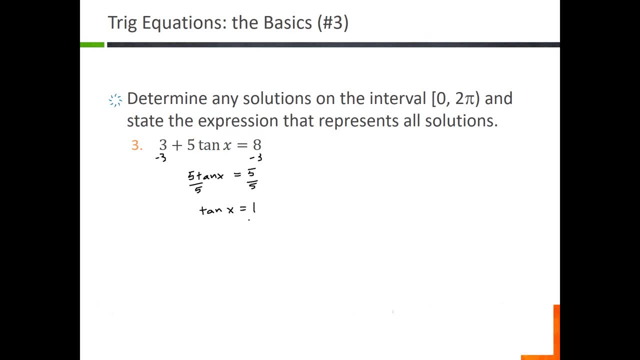 trig expression involving tangent and so now we want to think in terms of the unit circle So we want to know when is tangent 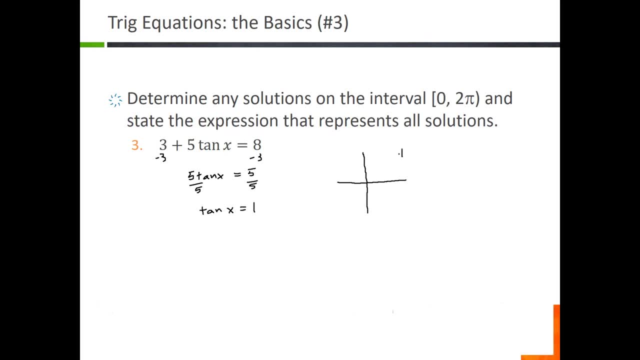 Equal to 1 well we know tangents positive in the first and the third quadrant Since we have a positive 1 we want it to be positive and Remember tangent is Y over X and so we want the points where the Y and the X coordinates are the same So in the first quadrant again, just using our unit circle. That's at PI over 4 In the first quadrant and then in the third quadrant That would be 5 PI over 4 so there's two answers between 0 and 2 PI so We would have X is equal to PI over 4 comma 5 PI over 4 and you can write those separately X equals PI over 4 and then X equals 5 PI over 4 But you can kind of merge them together Again, this is the solution 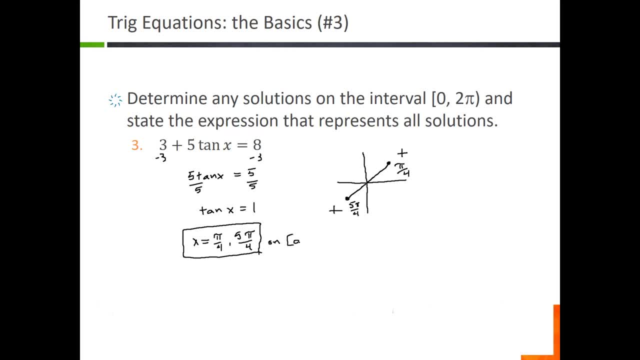 Those are all the answers on the interval from 0 to 2 PI So how do we express the? 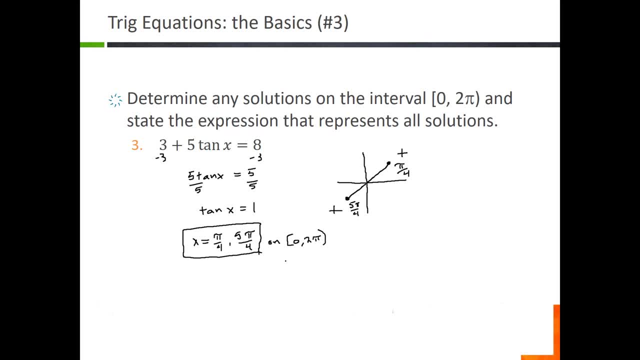 infinitely many solutions well with tangent we can kind of do this in two ways One we could take each of those solutions and add a 2 PI so X equals PI over 4 plus 2 PI K and then we could also say X is equal to 5 PI over 4 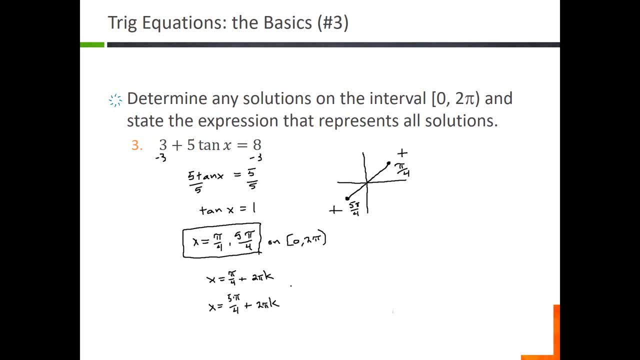 Plus 2 PI K. But there's a we have particularly with tangent and particularly in this case we have a better way of doing that okay if you remember with tangent instead of adding a 2 PI K there are actually two things that we I mentioned in that list of the process that we can follow there's two things I mentioned that we haven't kind of talked about here one is when we talk about tangent we only need to look at answers between 0 and PI and then the second part is that we're only going to add a PI K okay so for the two answers that we had PI over 4 and 5 PI over 4 we only need to keep PI over 4 we only need to keep the first one because that's the 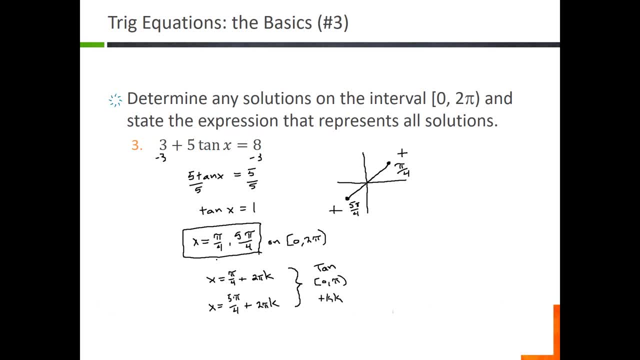 only one of the two that's between 0 and PI 5 PI over 4 is bigger than PI so we could have expressed so far this as X is equal to just 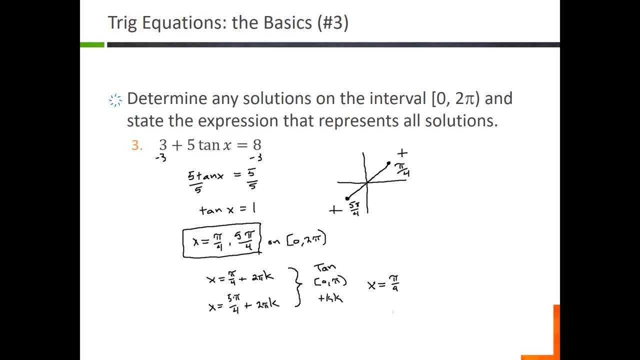 PI over 4 and then the second part is instead of doing plus 2 PI K we're just going to add in a plus PI K okay so why can we express our answer this way why 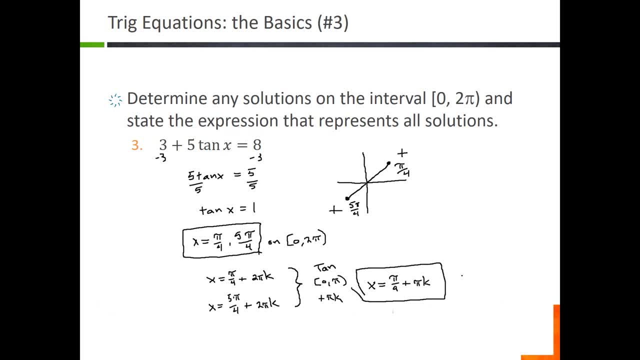 can we just express our infinitely many solutions using the one expression for tangent and then the plus PI K well let's see if we can do that okay so we can just keep going okay well to understand that let's go back to the graph to our unit circle we know one is that PI over 4 and the others at 5 PI 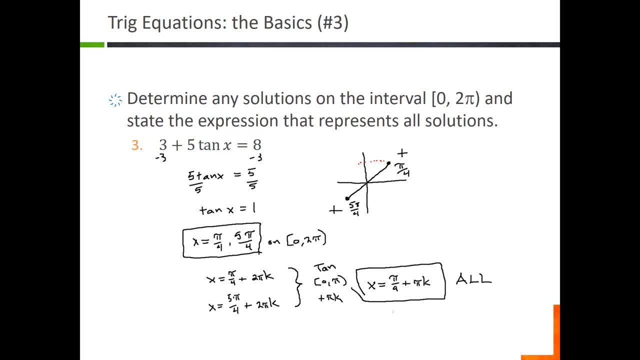 over 4 well how far is it from if we follow the unit circle from PI over 4 to 5 PI over 4 okay so from a 1 PI over 4 to a 5 PI over 4 is a distance of 4 PI over 4 which turns out to be pi so that's what we're going to get if we do this we're going to get pi over 4. OK, so from a 1 pi over 4 to a 5 pi over 4 is a distance of 4 pi over 4 which turns out to be PI. So, I'm going to pause this and I'm just going to do a little bit of a process here here and then we're going to take a few more minutes and then we're going to start working with each other. 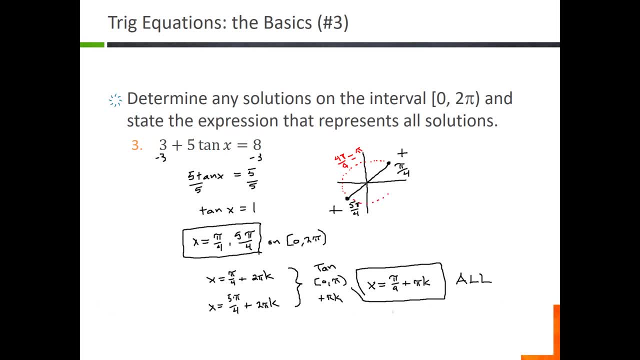 And so how far is it from 5 pi over 4 back to where the point at pi over 4 would be? If we kept going counterclockwise, this would actually be 9 pi over 4 if we kept going around, if we kept counting, so we'd have 9 pi over 4. But it's still a distance of pi. And if you look at these, these two points are exact opposites across the origin from each other. They form a 180-degree angle, so they're a straight line. So that means it's always a distance of pi from the first point to the second, from the second to the third, or coterminal back to the first, from the first to the second, from the second to the first, from the first. And so we can just keep going around and around and around. 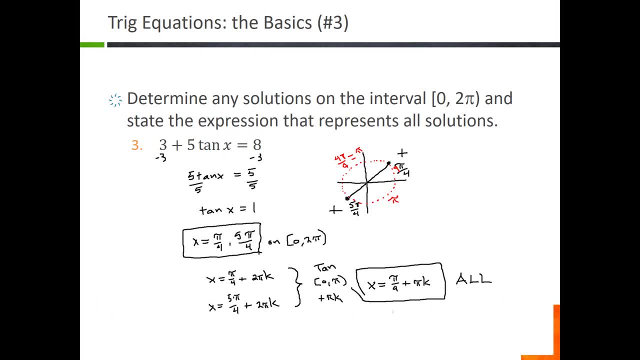 By starting at the first point and then adding a distance of pi, you get to the second. And once you add another pi, you get back to the first point, or coterminal to the first point. So. 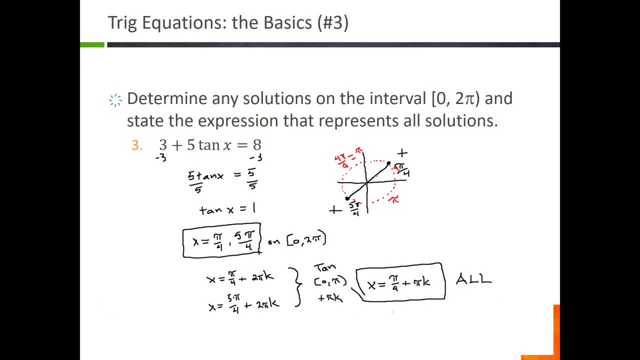 That pi, because tangent only has a period of pi, we don't need to include all the answers. If we did, we'd actually have a sort of, we would be repeating answers. So we only need to list any answers between 0 and pi, and then do a plus pi k for each of those. All right, let's look at another example. 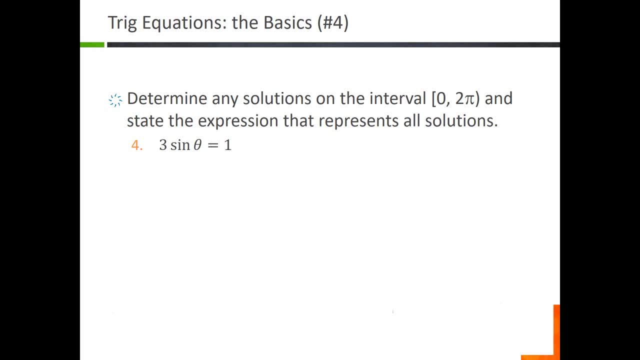 So we have 3 times the sine of theta is equal to 1. 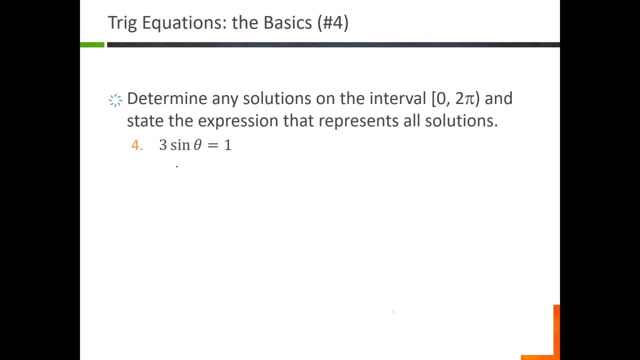 So let's just do algebra again here. To get sine by itself, we're going to divide both sides by 3. And so we get the sine of theta is equal to 1 third. 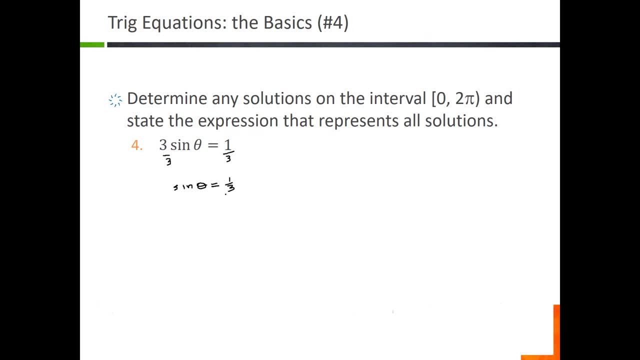 And so at this point, we need to stop and think. So we have it simplified as far as we can go. 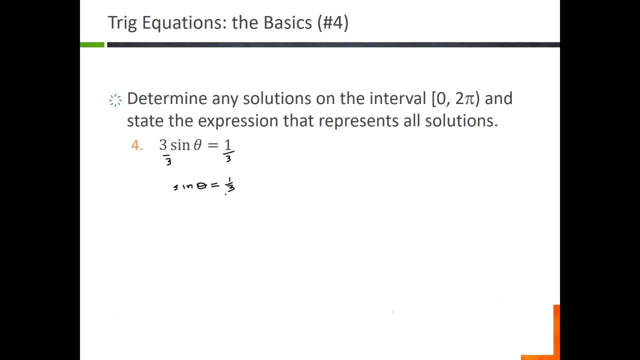 But 1 third is not one of our unit circle angles. So how do we go about finding when sine is equal to 1 third? Well, let's pause on that. 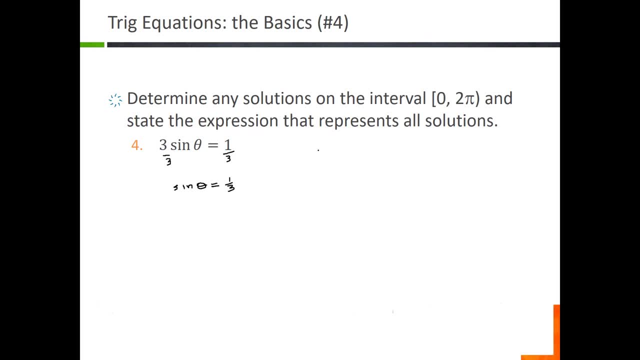 For a moment, and let's think about where, roughly, where it will equal 1 third. 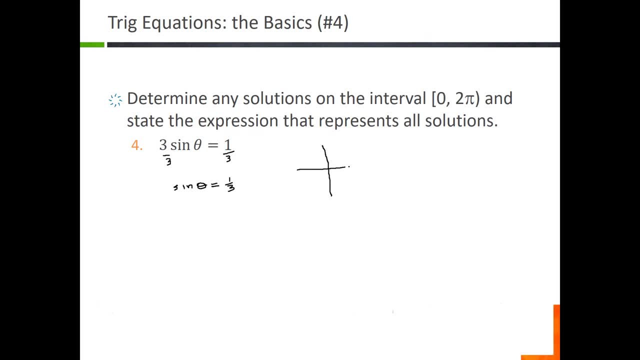 So let's talk about the unit circle here. Where is sine positive? Well, it's positive in the first, and it's positive in the second. 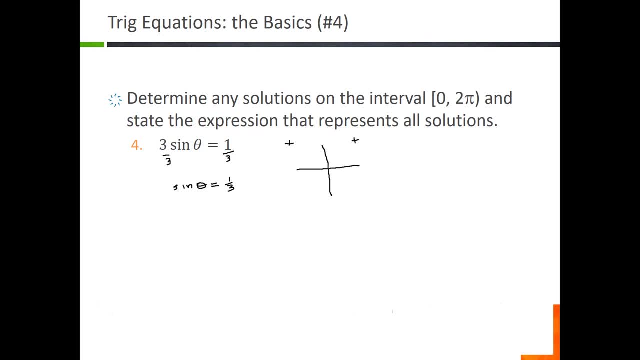 And remember, sine represents the y-coordinate. So somewhere on our unit circle, in the top half of the unit circle, we have two points. One in the first quadrant, and one in the second quadrant. Where the y-coordinate is equal to 1 third. Okay? So how do we find that angle? 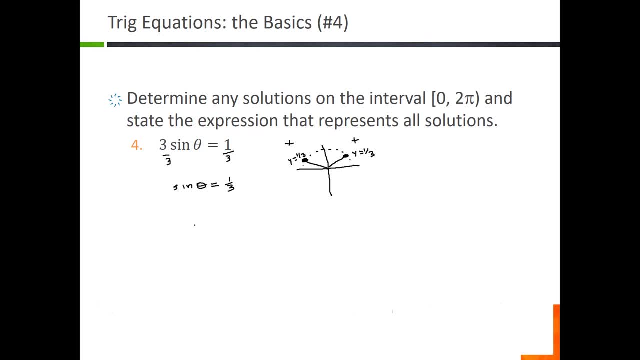 Well, we've looked at a method to do this a week or a couple weeks ago. 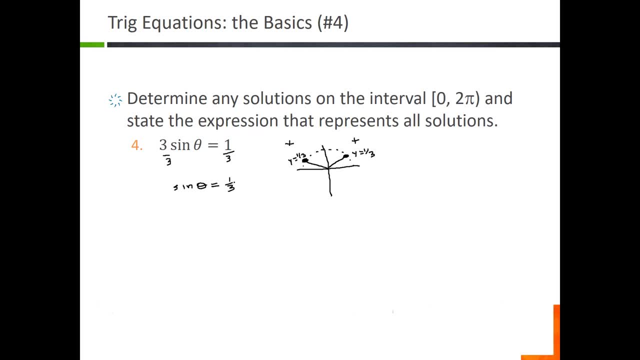 If we're trying to find the angle, and it's not a unit circle value, we can use inverse sine. So we can solve for theta by communicating. 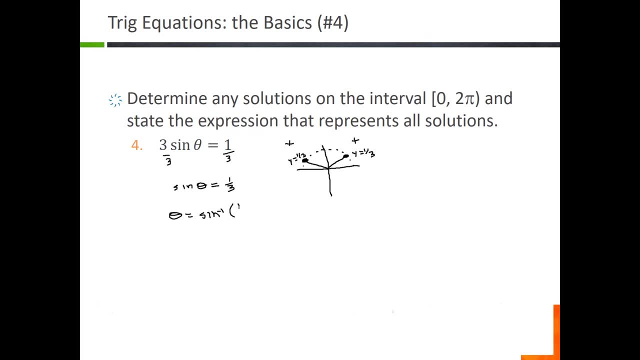 So we can compute the inverse sine of 1 third. Okay? 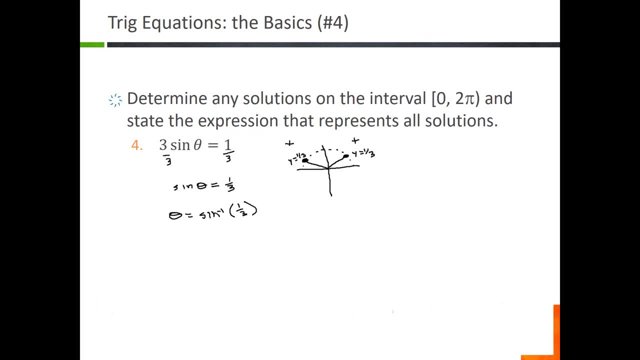 So again, inverse sine represents the angle whose sine is equal to 1 third. Which is what we're trying to compute to begin with. 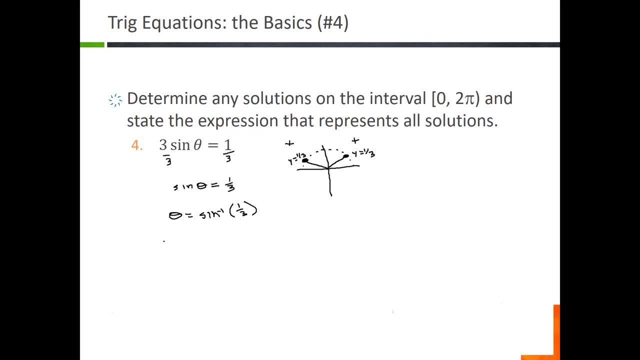 Now, since 1 third is not a unit circle angle, we're going to have to do this using our calculator. So if we type in the inverse sine of 1 third. 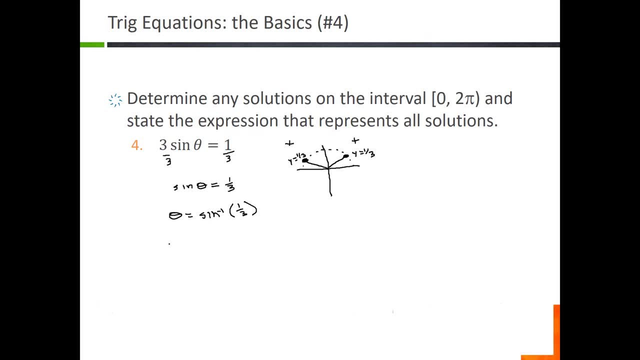 And we compute that, let's make sure that we are in radian mode. 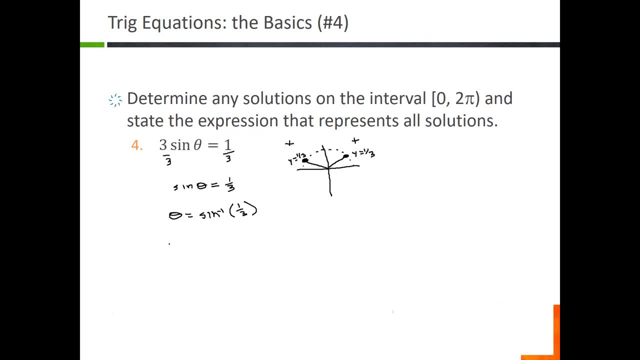 We don't want to be in degree mode, we want to be in radians. The inverse sine of 1 third is 0.3398. 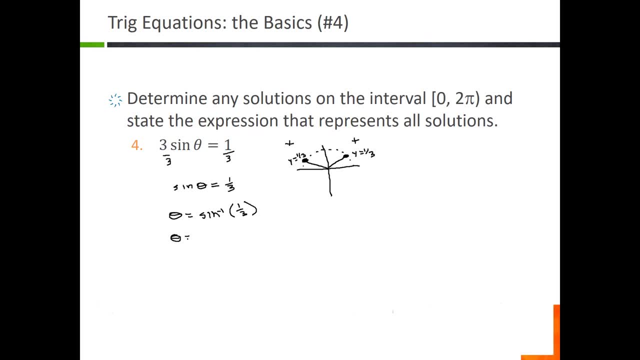 So we get theta is equal to 0.3398. And it's in radians, so I'm not going to put the degree symbol. Okay? Now here's the thing. Okay? 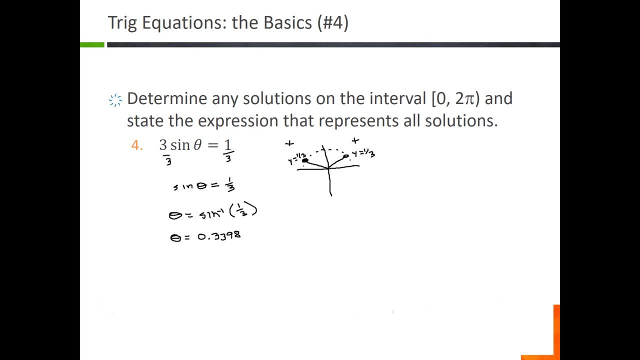 How many solutions are there supposed to be? There's supposed to be two. 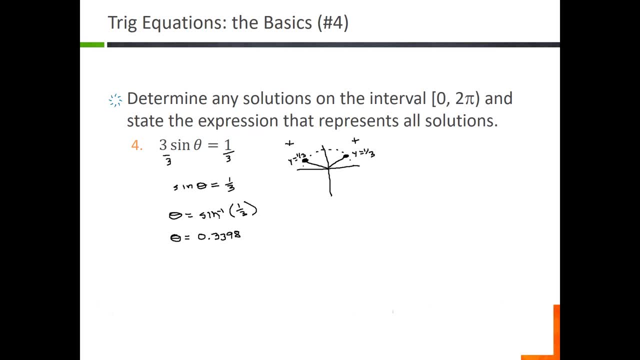 One in the first, one in the second quadrant. But when you do inverse sine, remember inverse sine is only going to give you an answer in the first or the fourth. 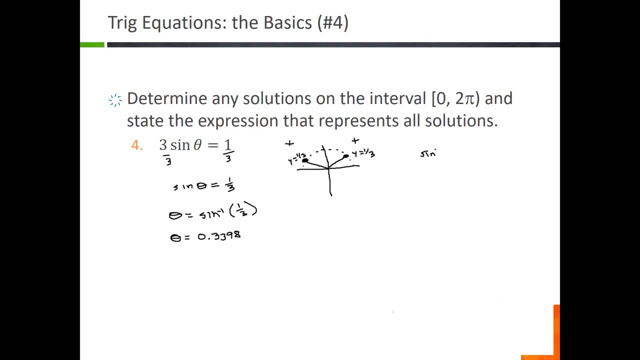 Remember when we compute inverse sine, our angle, our angle is going to be between a positive pi over 2. 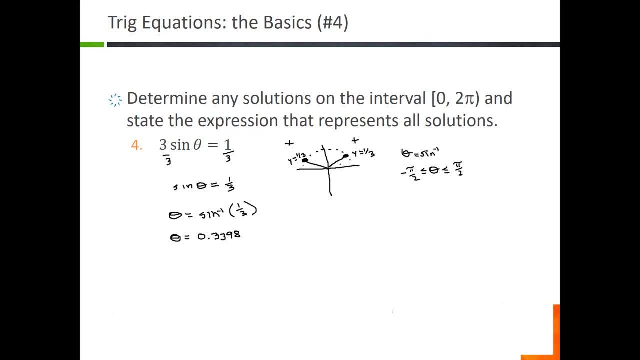 And a negative pi over 2. So it's actually going to be in the first quadrant as a positive value, or it's going to be in the fourth quadrant as a negative value. So since this came out to be a positive 0.3398, I know that it's in the first quadrant. 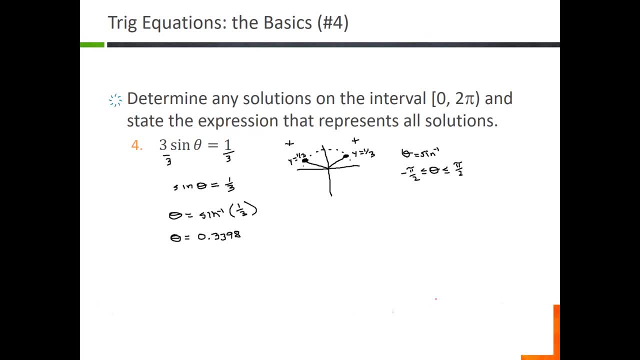 So how do we find the second angle? Well, let's think about what that 0.3398 represents. 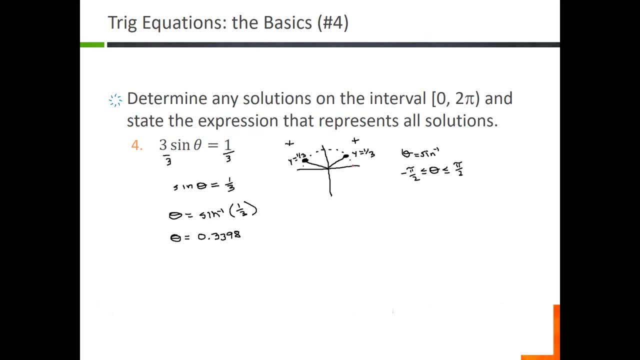 It is the angle from the x-axis to the point on our side. Okay? Okay. Okay. So this is our unit circle. So this angle here is that 0.3398. 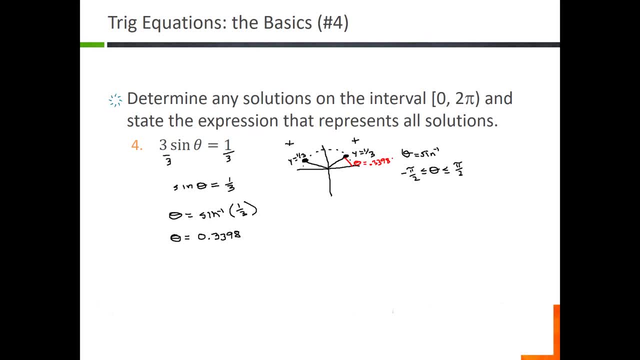 Okay? And if you remember the way we developed the whole unit circle, that is an acute angle. 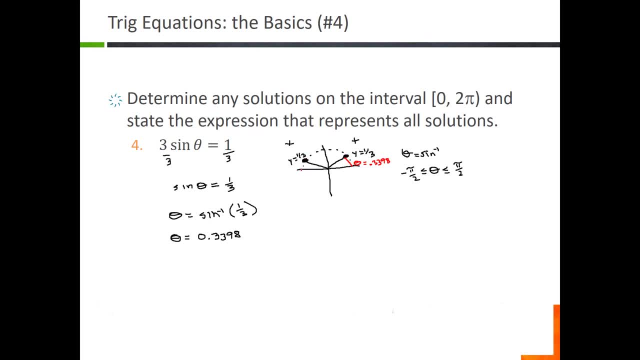 And so the second angle in the second quadrant, it has to have an acute reference angle that also extends down to the x-axis. 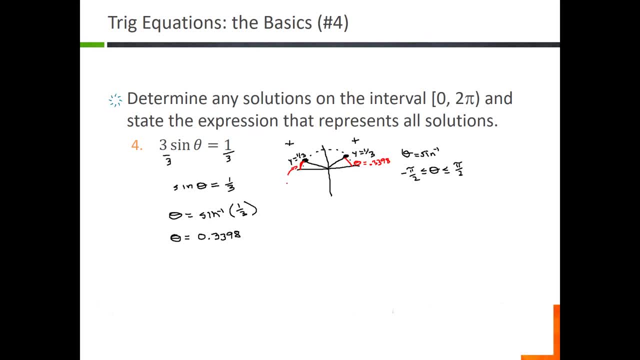 And that angle there is also 0.3398. Okay? Okay. 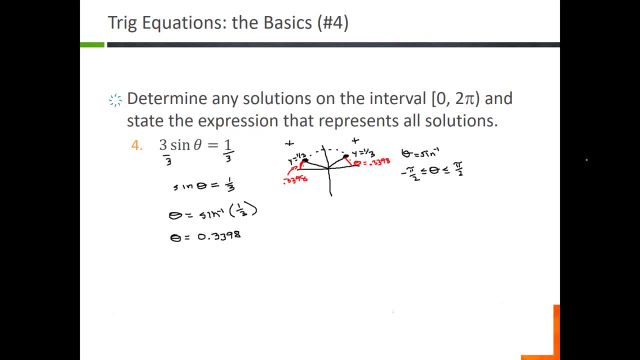 So how do we find the total angle? Well, the total angle would rotate from the x-axis to our actual point. Okay? And that's the angle we're trying to find. 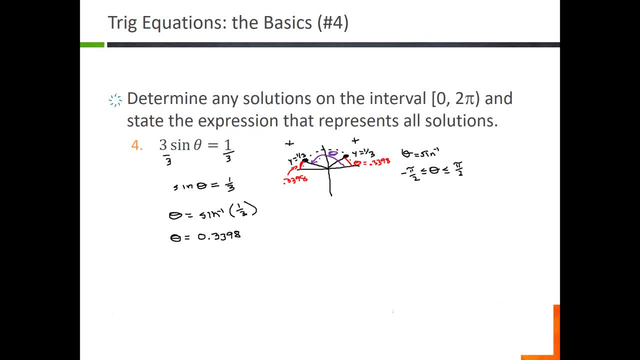 So theta, theta is the rotation, we'll call it just theta again. Theta is the rotation from the x-axis to our second point. 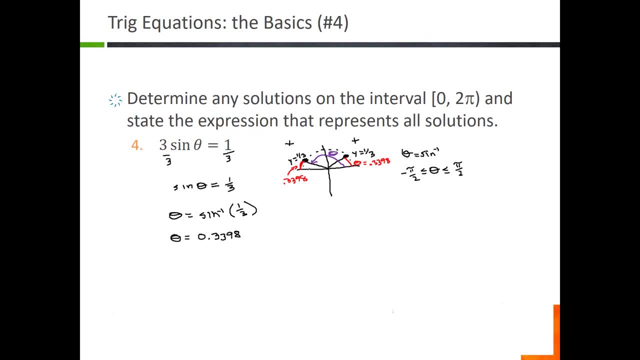 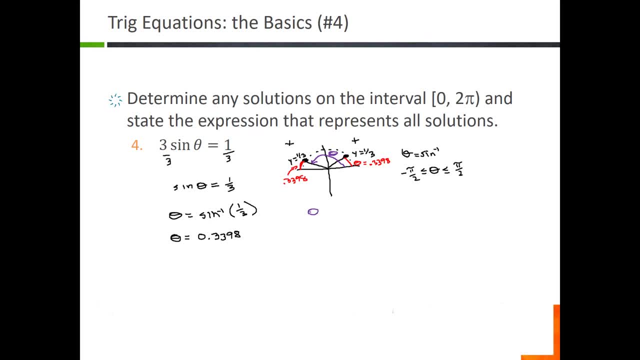 So theta created by theta is 0.3398. So that means if we did theta, our second angle, plus 0.3398, what is the total of that rotation? 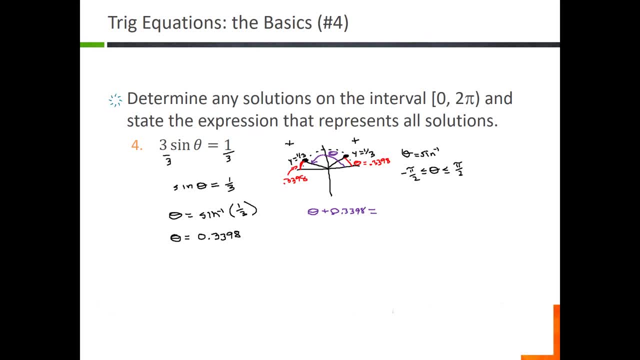 So if we rotated from the positive x-axis, we rotated a distance of theta to the second point. And then we rotated 0.3398. Where do we end up? Believe it or not, it Amazing. 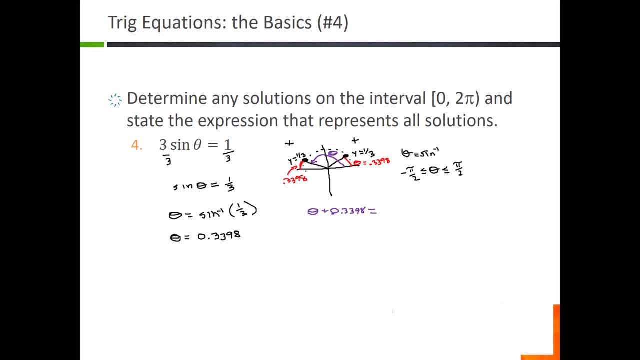 Where do we end up? We'd end up on the negative x-axis. So what rotation goes from the positive x-axis all the way around to the negative x-axis, which is half the circle? It's a distance of pi. 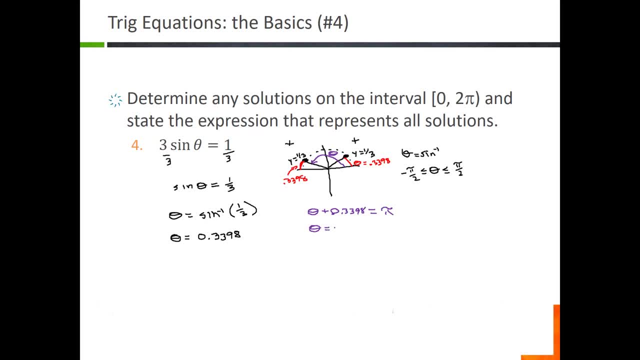 So if we solve that for theta, we're gonna get theta is equal to pi minus 0.3398. And we can compute that on our calculator. 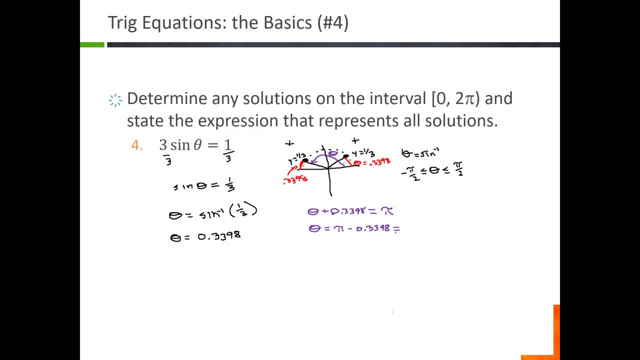 So if we compute pi minus 0.3398, we're going to get 2.8018, depending on how you round it. 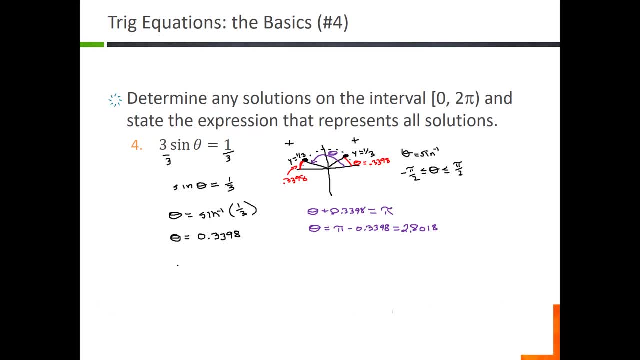 So that gives us our second answer. We know theta will have two answers, 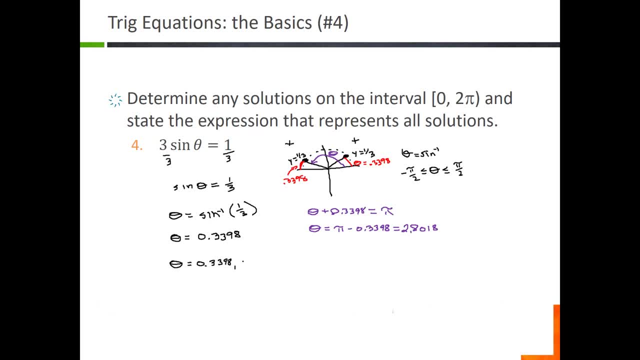 Either 0.3398 or 2.8018. 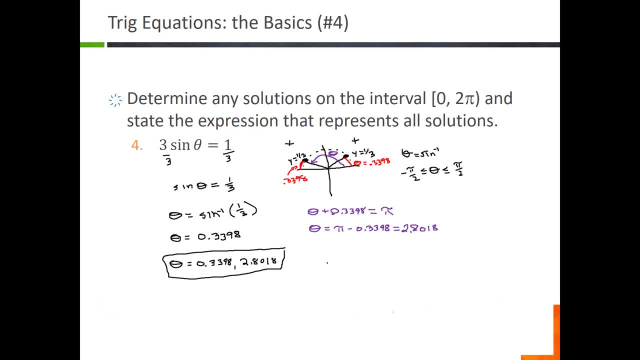 And again, those are the solutions only on the interval from zero to two pi. 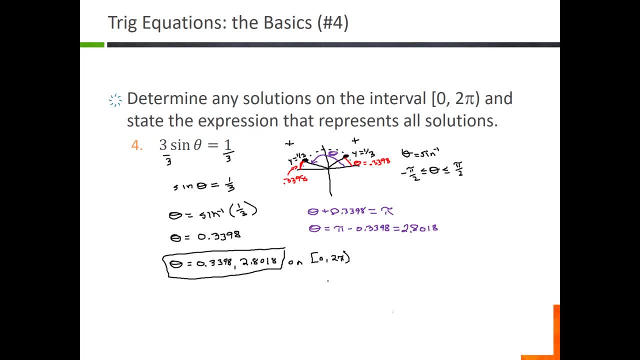 Okay, so how do we find all the solutions? Well, we do it the same way we did before. We're gonna have to write for each of the two answers, we're gonna have to add a plus two pi k. 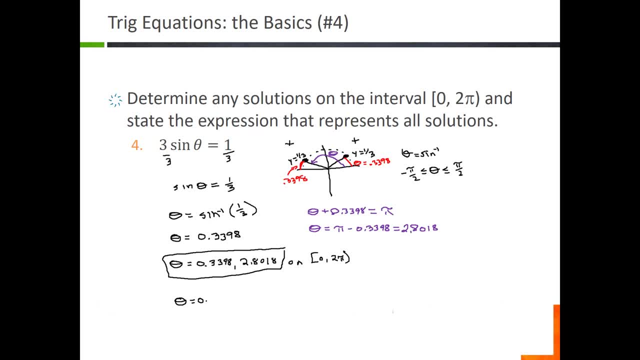 So we're gonna have theta is equal to 0.3398 plus two pi k. 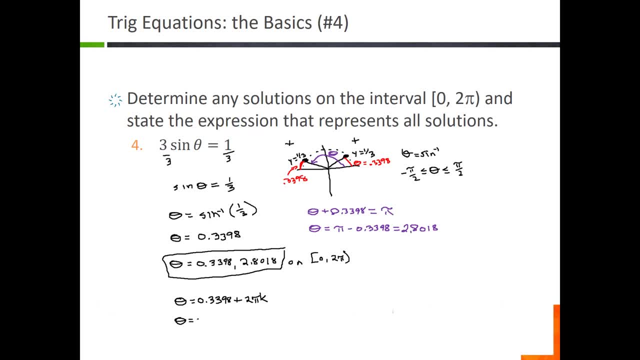 And we're also gonna have theta is equal to 2.8018 plus two pi k. 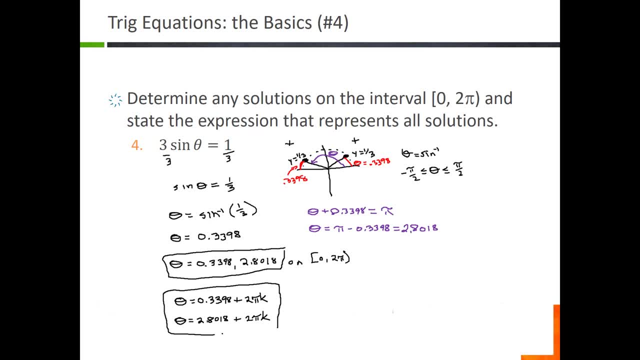 And together, these two statements represent the infinitely many solutions as we rotate around and around and around the unit circle. 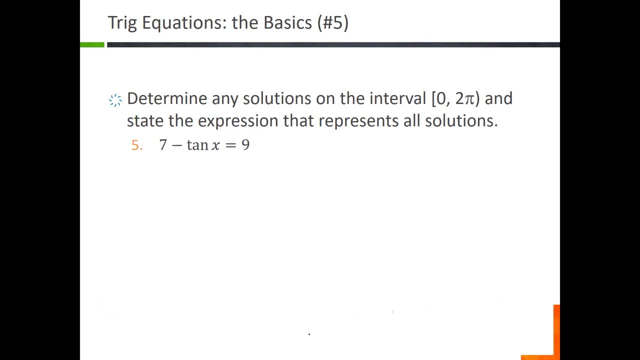 Let's look at another example, this time involving tangent again. So same process, we want to find all the solutions on 0 to 2 pi, and we want to state all the infinitely many solutions. So for this example, we have 7 minus the tangent of x is equal to 9. So to get tangent by itself, we're going to subtract a 7 from both sides. So we're going to be left with a negative tangent of x is equal to 2. And then we want to multiply both sides by negative 1, just to move that sign over. So we have tangent of x is equal to a negative 2. All right, so we've got it simplified. 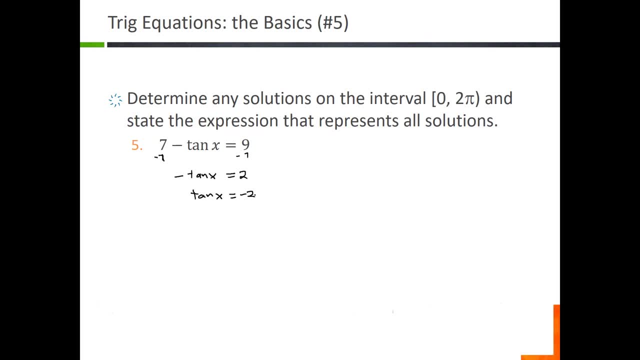 So we're ready to use the unit circle. If we can, so how do we find when tangent of x is equal to a negative 2? 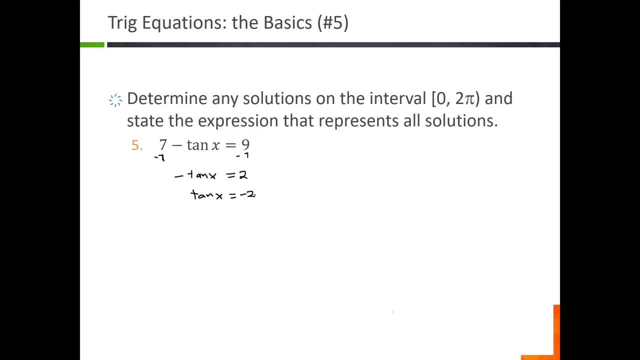 Well, is that a value on the unit circle? And the answer for that is no. 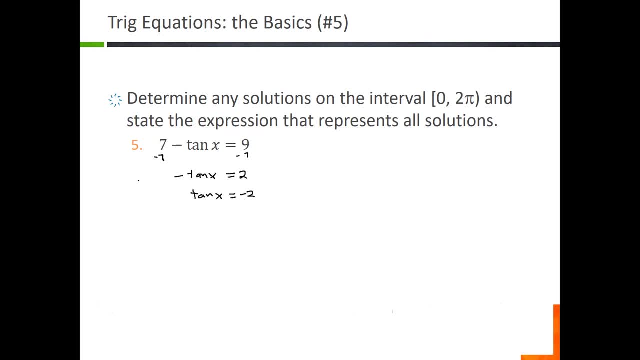 So this is not on the unit circle, at least not one of our exact values. 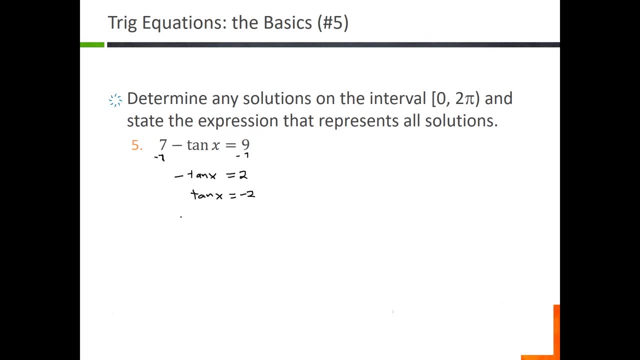 So we're going to have to use, just like we did in the last example, we're going to have to do an inverse tangent. So x is going to equal the inverse tangent of a negative 2. So if we compute the inverse tangent of a negative 2, we're going to get x is equal to a negative 1.1071. And that's rounded to four decimals. 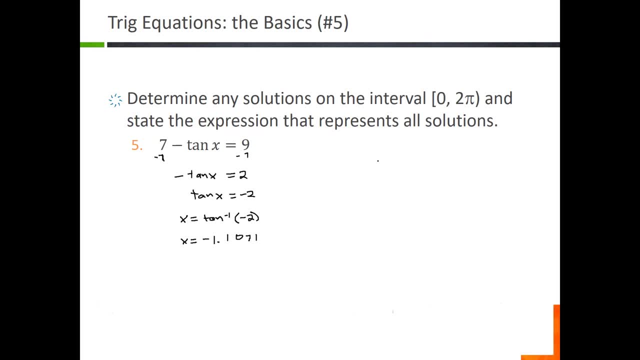 Okay, so how many answers are there between 0 and 2 pi? Well, let's think about where tangent... where tangent is positive and negative again. So do we want to know where tangent is positive or where tangent is negative? Well, based off of our simplified equation, we have tangent of x is equal to a negative 2. So we want to know where is tangent negative? Well, it's positive in the first and the third, which makes it negative in the second and the fourth. 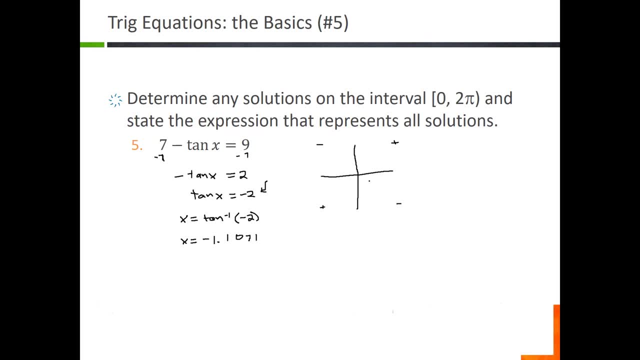 So this negative 1.1071 is an angle, which makes it negative in the second and the fourth. So this negative 1.1071 is an angle, which makes it negative in the fourth quadrant, 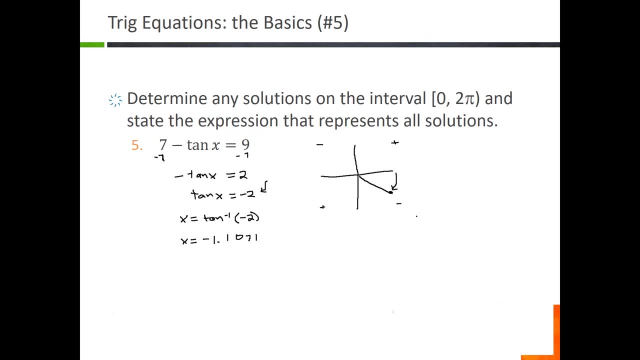 and since it's negative, it is rotating clockwise down into the fourth quadrant. 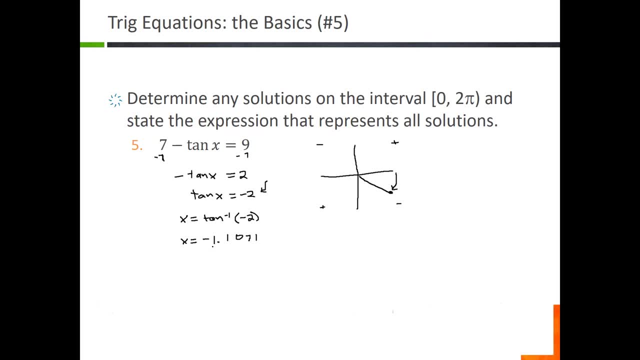 Okay, now, and this negative 1.1071 it's not even itself on the interval from 0 to 2pi. 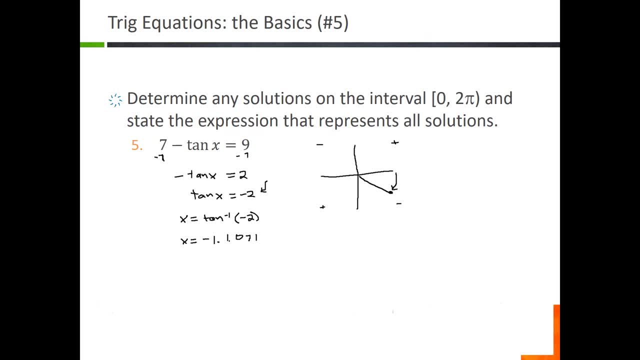 So that's not actually gonna be one of my final answers. It's not within the interval that we want. 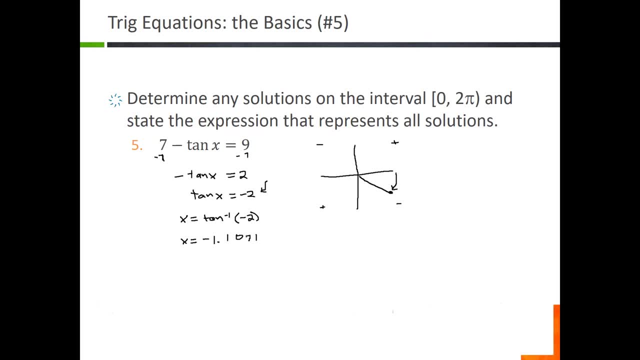 So how do we find the answers that are? Well, this is going to involve the nice answer, 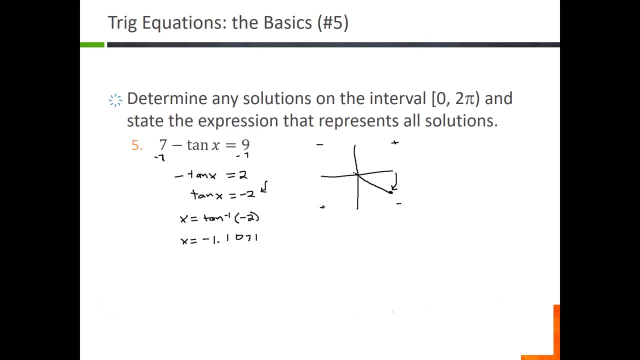 the quick answer, nice thing with tangent is we just need to go halfway around the circle. So if you're in the 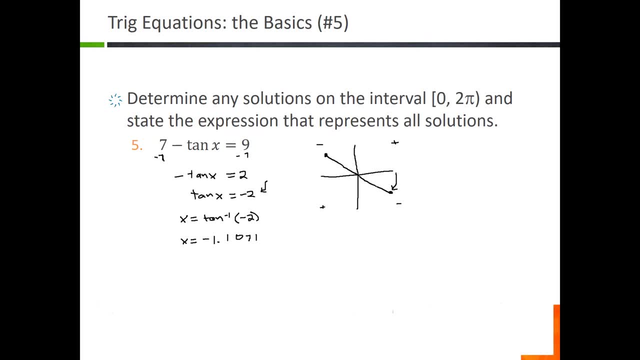 fourth quadrant you can get into the second quadrant by adding pi because it makes 180 degree angles. So if we rotate a distance of pi from my given answer I will end up in the second quadrant and it will actually be positive now. And so how do we find the second answer that's between zero and two pi? Well again the nice thing about tangent take the answer we just got and add another pi to it or add two pi to our original answer. Okay so again it's always just rotating around half the circle. So to find our first answer let's take our the answer we got from our inverse tangent a negative 1.1071 and let's add pi to that. 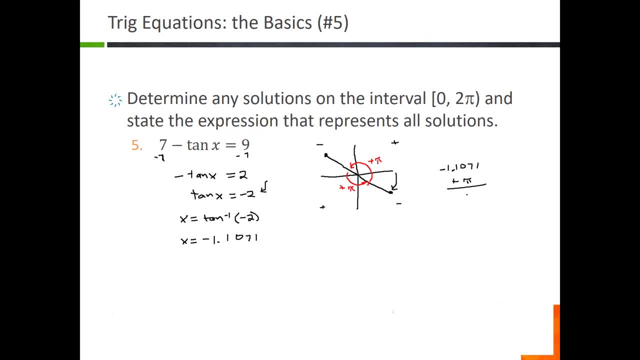 And if we do that we will get 2.0344 and again that's rounded to four decimals. So this is the answer in the second quadrant. Well how do we get the fourth quadrant? We're going to add another pi to that and that's going to give us 5.04. That's the answer in the fourth quadrant. Okay so what is one of my solutions between zero and two pi? So we know x would equal 2.0344 and we know it's also equal to 5.1760. So those are the two solutions that we get. 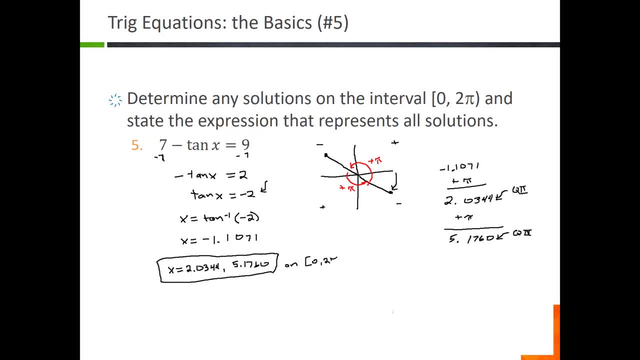 On the interval from zero to two pi. So again this was a little harder because the first answer we got that negative 1.1071 was not even one of the two answers we wanted to keep. It was we had to use it to get to the answers that we wanted because again this number negative 1.1071 is less than zero. 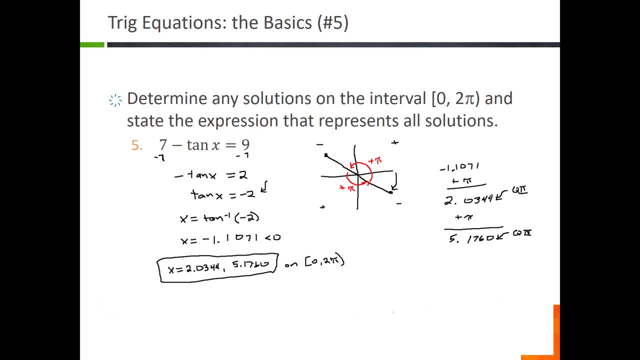 It's not between zero and two pi. So we have all the solutions from zero to two pi. So how do we express the infinitely many solutions? Okay well first again remember that our two answers the 2.0344 and the 5.1760 both of those are a distance of pi away from each other the way that we have this rotation going around. And we could rotate in the other direction too but we know they're a distance of pi. And we also know that when we show our infinitely many answers we only need to do a plus. Pi k. We can list both of these out and do plus 2 pi k but we want to have a nice clean answer. So we only need to keep that first one. So x is equal to 2.0344 plus pi k. And so that expresses all of our solutions. We don't need to keep both if we do the plus pi k because it's. 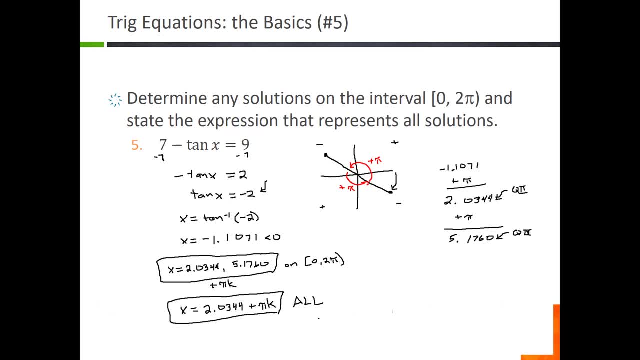 You're always adding a Pi k. Pi k. Just like we found the 2.0344 and the 5.176 we're just adding pi over and over and over again. 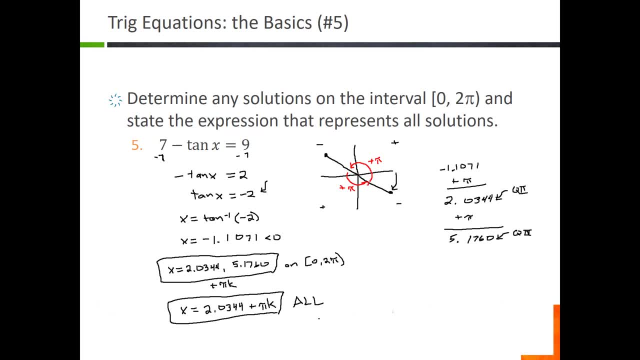 So just using the one answer will then generate all the other answers that we need. 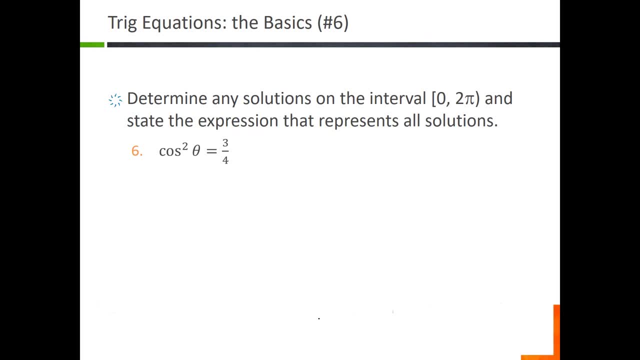 All right let's look at one more answer with just kind of basic algebra. But this one's a little different. So we have cosine squared of theta is equal to three-fourths. 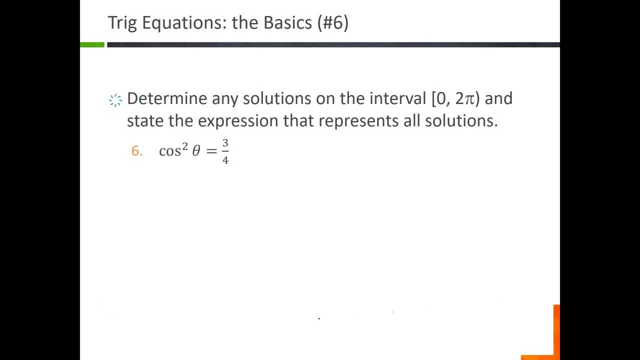 So it's a little different because we have a square in it. Now when you see the square again you might be tempted to use an identity right. 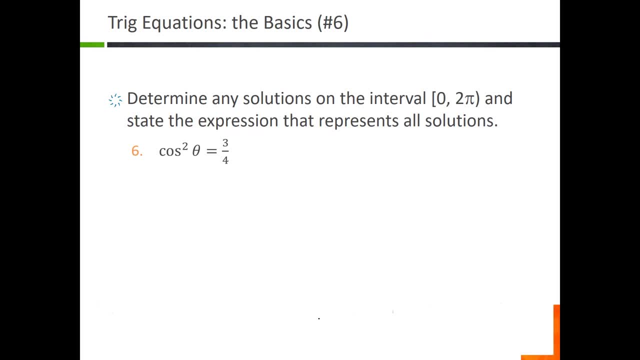 We have the Pythagorean identity. We have the reduction in identities but we're not going to worry about identities right now. 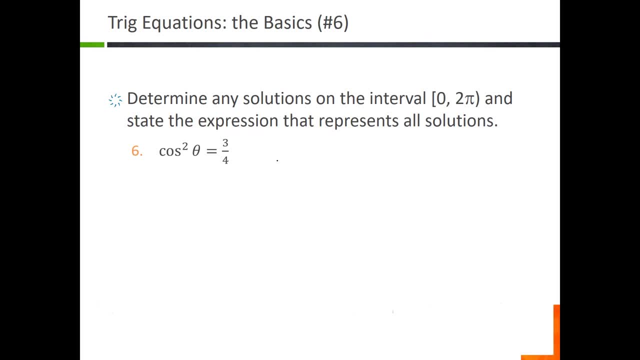 We're just going to do some algebra. So let's just think for a moment. 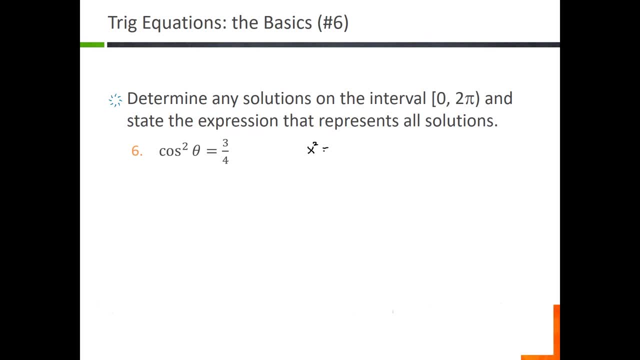 If I had the equation x squared is equal to three-fourths how would you get x by itself. Well you'd take. the square root of both sides of your equation and so we would get x because the square root of x squared is just x equals the square root of three-fourths. Now and one other thing to keep in mind when you take the square root of both sides of the equation you will get a plus or minus and the square root of three-fourths you could simplify it a plus or minus the square root of three then divided by two because the square root of four is the two. So we get plus or minus root three over two as x okay. 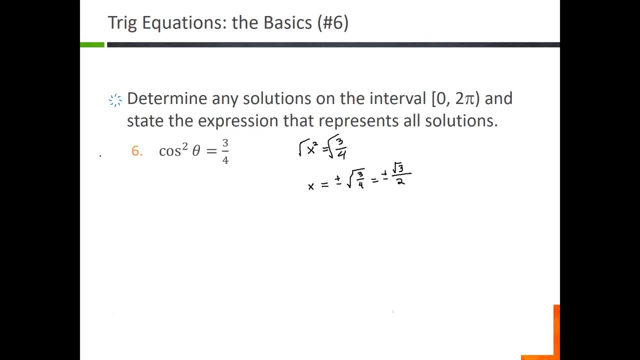 But again in our problem we're not trying to find x we're trying to find theta. So we have the cosine squared of theta is equal to three-fourths but same idea. We're going to take the square root of both sides and so that's going to leave us with the cosine of theta would be equal to plus or minus a square root of three over two. So pause for a second is square root of three over two one of our unit circle values for cosine? Yes it is. Okay so we can come up with exact values we don't need to use our calculator. And then we also need to think where is it positive and where is it negative because when we have this plus or minus we can actually break this apart. We have two equations technically. We have the cosine of theta is equal to a positive root three over two. 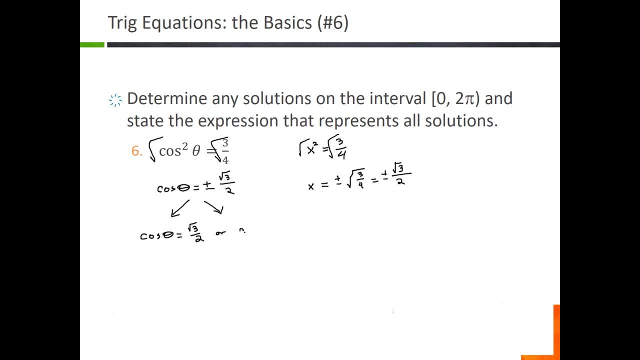 Or we also have the cosine of theta is equal to a negative root three over two. Okay so there's two different ways that are this plus or minus converts us into two separate equations and we need to come up with answers for both of those. 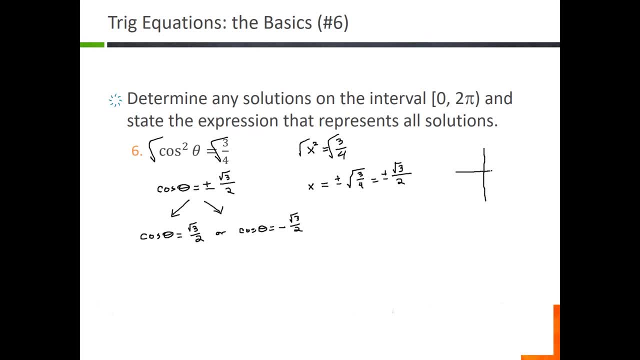 So let's go over to our unit circle and our quadrants. Where for first where is cosine positive? Again cosine is positive in the first and the fourth so it is negative. 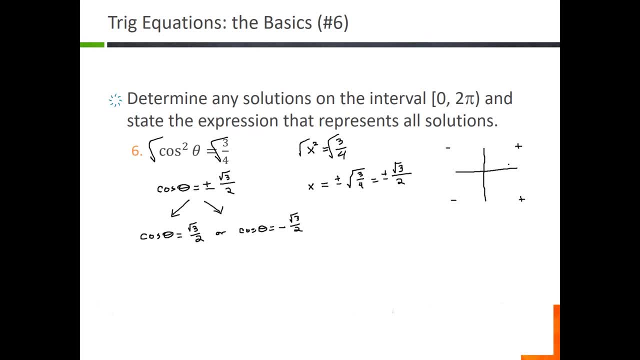 In the second and in the third. And when is cosine root three over two? It's at 30 degree angle which is pi over six. So we want the pi over six angles in the first and the fourth quadrant. So pi over six and then an 11 pi over six because that puts us another one down here in the fourth quadrant. So these are the positive two. We're also going to have one in the third or second and one in the third quadrant. So the pi over six angles over on the left side are going to be five pi over six and seven pi over six. So those are the four angles on the unit circle from zero to two pi that produce either a a cosine of either a positive root 3 over 2 or a negative 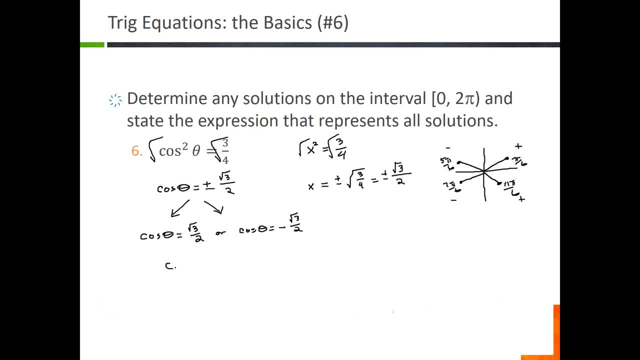 root 3 over 2. So that means theta is going to equal all four of these. So we're going to have theta is equal to PI over 6 PI over 6 7 PI over 6 and 11 PI over 6 so all four of these together represent the solutions on the interval from 0 to 2 PI all right so how do we then express the solutions for all solutions so how do we express the fact that there's infinitely many well it's cosine and so for cosine we're just going to take all four of these and put on a plus 2 PI K onto them so we're going to have four of these statements so we're going to have theta is equal to PI over 6 plus 2 PI K we're gonna have theta is equal to a graduate 5 pi over 6 plus 2 pi k. We're going to have theta is equal to a 7 pi over 6 plus 2 pi k and then we're also going to have theta is 11 pi over 6 plus 2 pi k. All right and so all four of these again all four of these together represent all solutions. 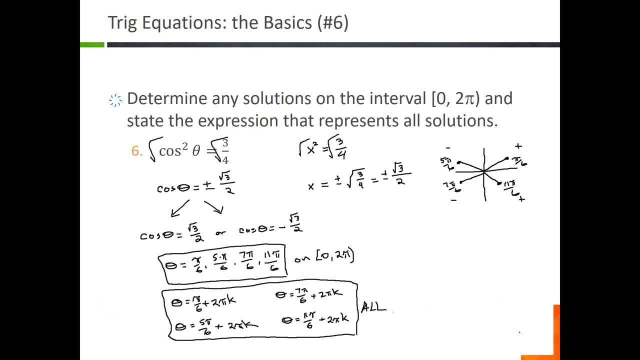 Now there is a little bit of simplifying that we can do here. 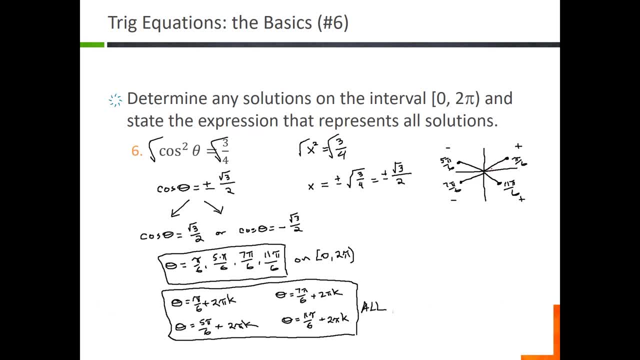 Notice that pi over 6 and 7 pi over 6 are opposite angles. They are straight across from each other. So that's means from pi over 6 to 7 pi over 6 is a distance of pi. Okay so if I had pi over 6 and I added pi to it I would get a 7 pi over 6 and if I took that 7 pi over 6 and I added a pi to it I would get at 13 pi over 6 but that's the same thing as pi over 6. So these are both just kind of like tangent these two the pi over 6 and the 7 pi over 6 they are distances of pi away from each other. And in sort of a similar way the 5 pi over 6 and the 11 pi over 6 are a distance of pi away from each other. Okay so if you had 5 pi over 6 and you added pi you'd get to the 11 pi over 6 and if you added 11 pi over 6 plus pi you would get a 17 pi over 6 which is the same thing. 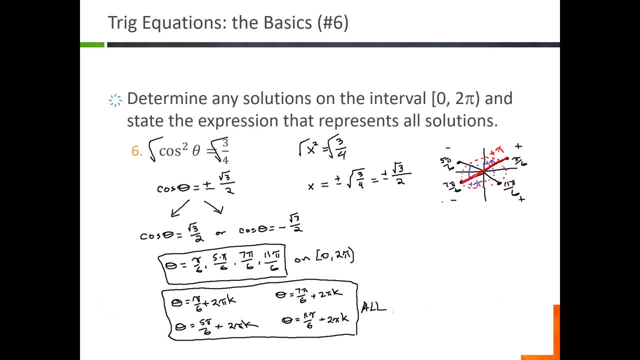 is 5 pi over 6. So what that means is we can take these four expressions that we had for infinitely many answers and we can merge them into just two answers. So the first one would take the pi over 6 and the 7 pi over 6 and we can write that as theta is equal to pi over 6 plus pi k and again it's a pi because that's how far it is between these two answers. So that takes care of the pi over 6 and the 7 pi over 6. The other two the 5 pi over 6 and this 11 pi over 6 those we could write based off of the 5. So we have theta is equal to 5 pi over 6 plus so how far is it from 5 pi over 6 to 7 or 11 pi over 6 it's a distance of pi. So again we're going to have a plus pi k and that takes care of the 5 and the 11 because again if you take a 5 pi over 6 and you add a pi that will give you an 11 pi over 6. Same thing with pi over 6 plus a pi that would give you the 7 pi over 6. So we could express instead of using all four answers to express the infinitely many solutions we could use just those two. 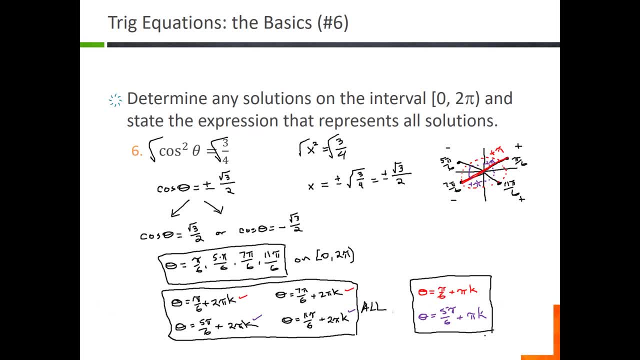 Now I don't care which way you do this like in the lab manual and stuff like that I think often times in the lab manual it will show you the second version of those four answers as two. But there's not necessarily a correct way to do it or not using just the plus pi over k is usually probably the simplest answer so if you're looking for the simplest answer that's what it would be. 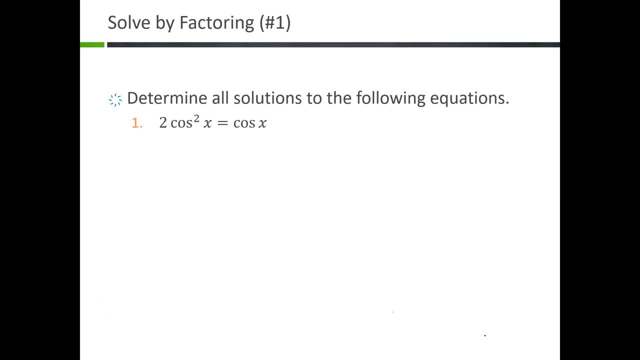 All right so let's look at a few examples involving factoring. So we're just going to look at finding all the solutions to the equation. So this first equation it's 2 cosine squared of x is equal to x and I really want to I really like this example because it's going to illustrate a common mistake that too many people make. To see what I mean by this let's look at this as just a simple algebraic. 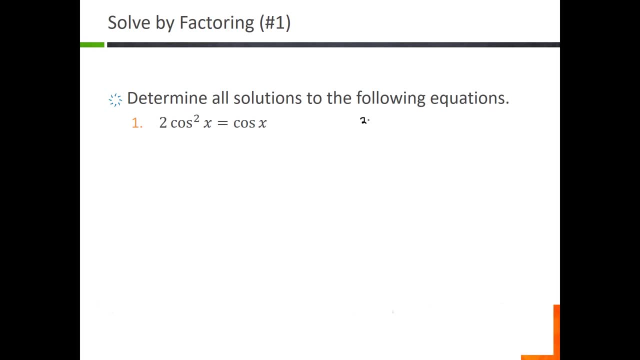 Equation so let's get rid of the cosines. What if we just had 2 x squared is equal to x and again sort of a common mistake people are going to make is when they see an x on both sides of the equation they're going to divide both sides by x which on the right side gives you a 1 and on the left side the x is reduced down a little bit so you're just left with a 2x and then solving for x gives x equals one half. 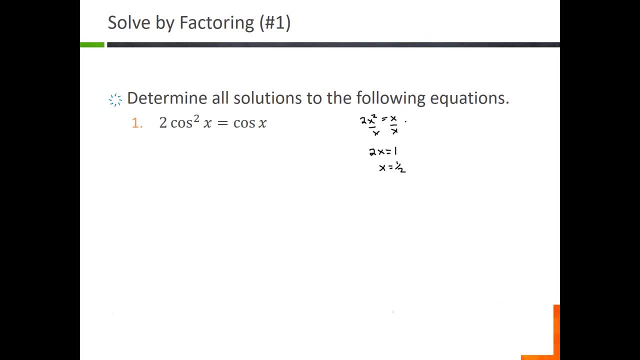 So if you were to plug that half into the original equation it would actually work. Two times a half squared which a half squared is a fourth two times a fourth is a half so it will actually work. But there's a one more number that will also work in this equation. 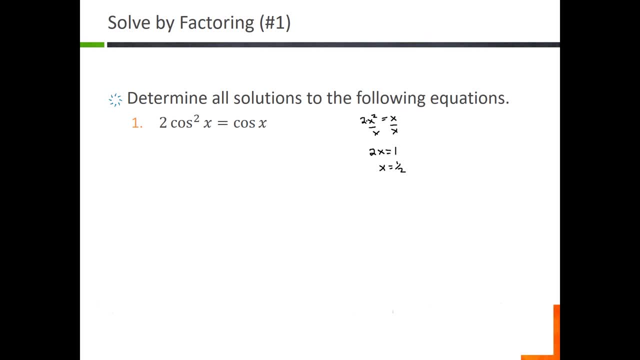 If I plug zero in for x I'll get two times zero which is zero is equal to zero. Okay. 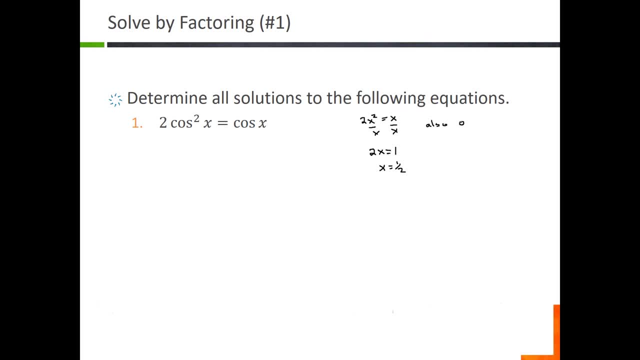 So we also need to have. A second solution and that's zero equal to zero. So if x is equal to zero we get a solution. 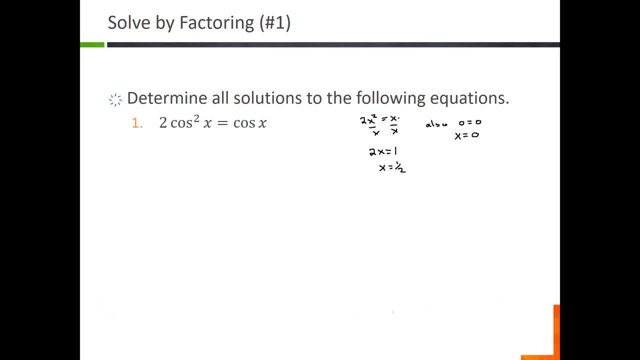 So the point being here is that just because we have an x on both sides of the equation we don't want to divide by x. Okay. Because we and it could be possible that we're dividing by a zero. And if we do that we're going to lose that zero. So if we divided by x we would have lost x equals zero as one of us as one of our solutions. Okay. 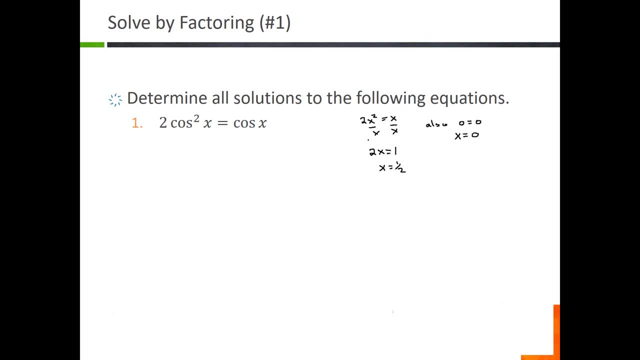 So the better approach to solving this kind of equation is don't divide. So instead we want to take two x squared is equal to x and we want to subtract the x to the other side. So that means we're going to have two x squared minus x is equal to zero. And now instead of dividing I can factor which is a sort of division but we're not technically dividing it out. So if I pull out an x I'm going to have x times the quantity two x minus one. And we know from algebra if you multiply two expressions and you get zero then we know one or both of those equations one of those parts is equal to zero. 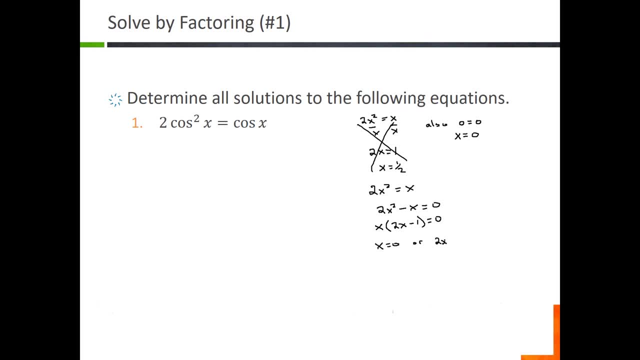 So either x equals zero or we have two x minus one is equal to zero which if we solve that for x we will get the half. 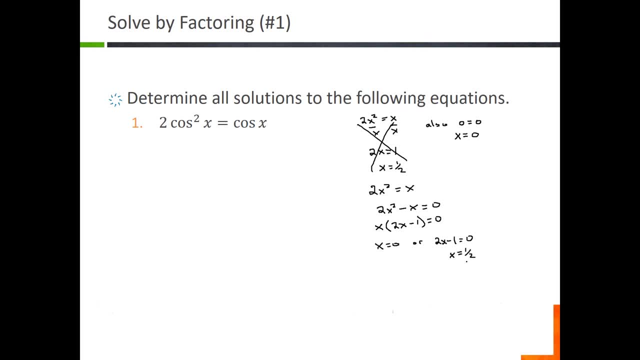 So by doing it using a factoring approach. We do end up getting both the half and the zero. 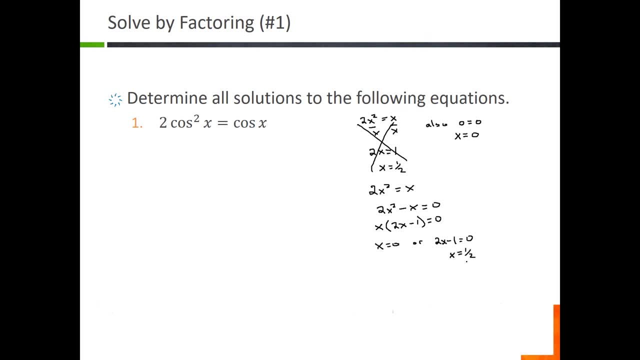 So when we see equations like two cosine squared x is equal to cosine x we don't want to think division we want to think factor. 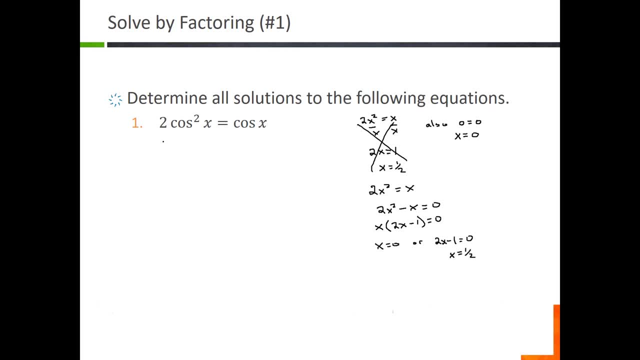 So let's go ahead and work through this problem using our cosines. So we have two cosine squared x is equal to cosine x. So instead of dividing we're going to pull that cosine x over. 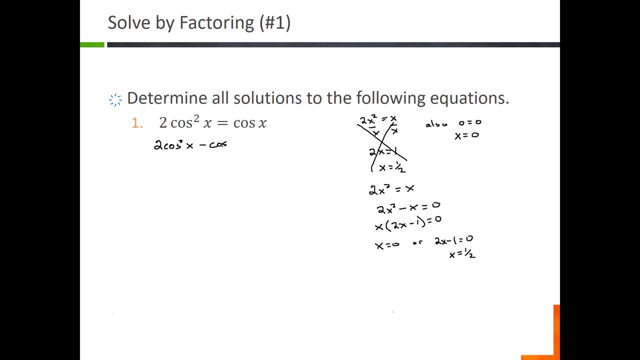 So it's two cosine squared x. Minus a cosine x is equal to zero and we're going to pretty much follow the same algebra. We're going to pull out a cosine x. When we factor that out we're going to be left with a two times the cosine x remaining and then minus a one. And again all that's equal to zero. So two things multiply to give you a zero. That means one of them or both of them is zero. So cosine x is equal to zero. 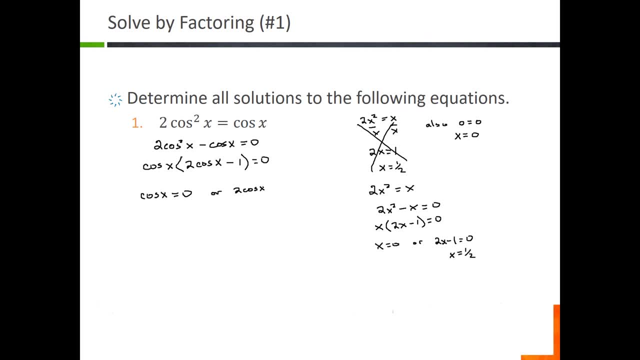 Or. Two cosine x minus one is zero. 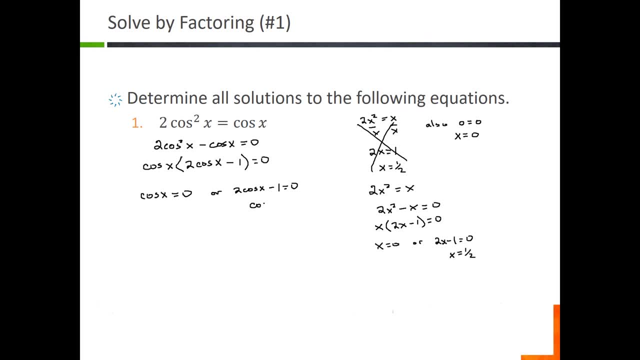 Which the two cosine x minus one equals zero is going to turn out to be cosine of x is equal to a half. 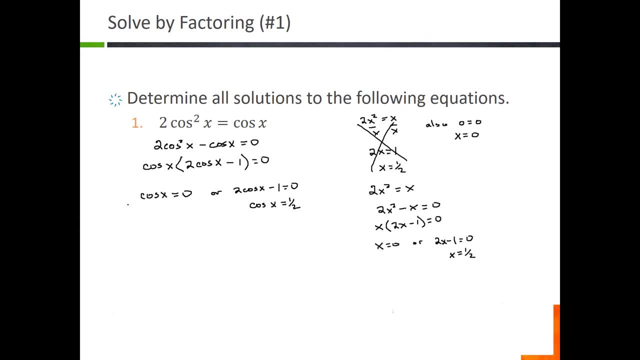 So we have basically two equations here that we need to solve for x. We have the cosine of x equals zero. And we have the cosine of x equals a half. So we need to find all the solutions for both of these. 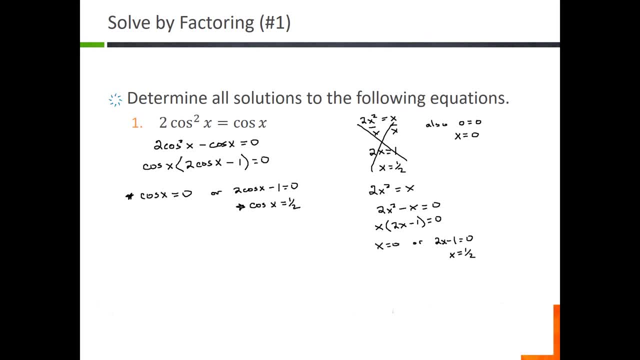 So let's go ahead and start with the cosine of x equals zero. 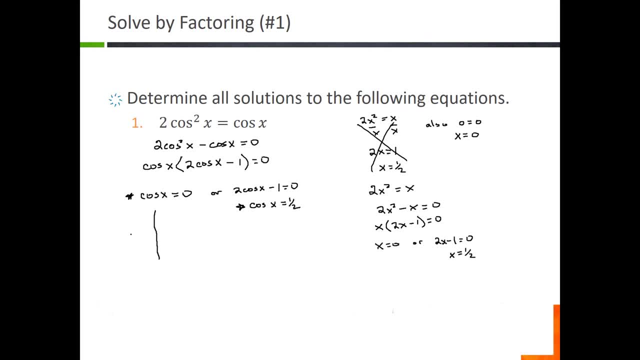 So on the unit circle where is cosine equal to zero? So remember cosine is the x coordinate on the unit circle. So that's the two points on the y axis. So zero one and zero negative one. So at zero one that is an angle of pi over two. And at zero negative one that's an angle of three pi over two. So those are both between zero and two pi. And so we can express all of our solutions as pi over two plus two pi k. And x equals three pi over two plus two pi k. 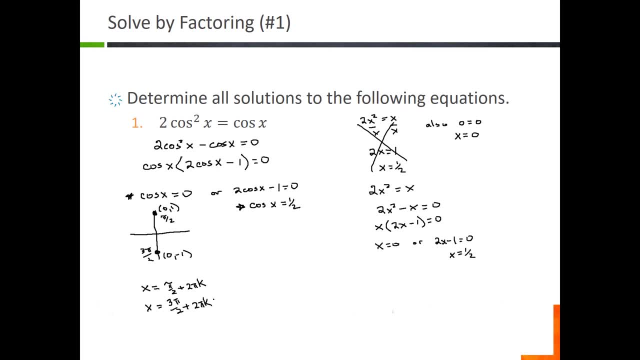 All right. So those are the two answers. The two expressions that we get. 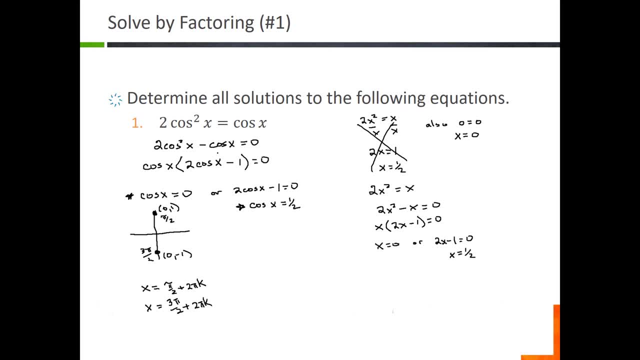 For cosine x equals zero. And then let's look at the cosine of x is equal to a half. 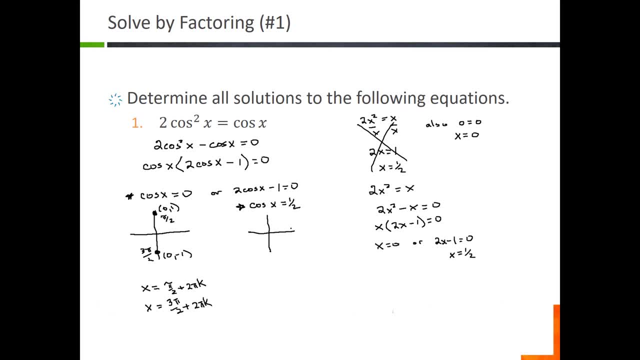 So where is cosine equal to a half? Well remember again go through the process. Cosine is positive in the first and the fourth quadrant. And we know in the first quadrant cosine is a half at pi over three. 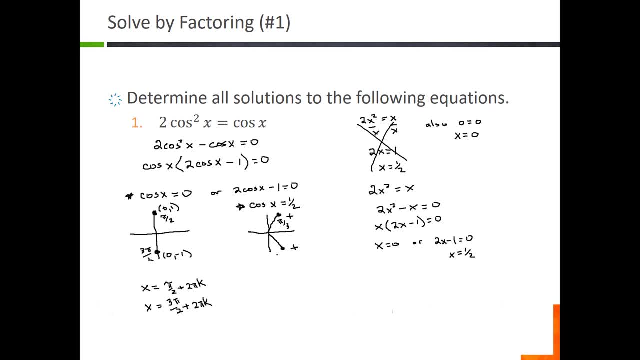 So what is the pi over three angle in the fourth quadrant? Again using our unit circle. It's going to be a five. 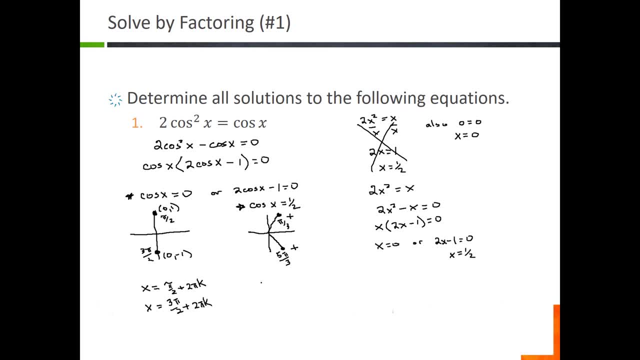 Five pi over three. So those are the two angles that we get. 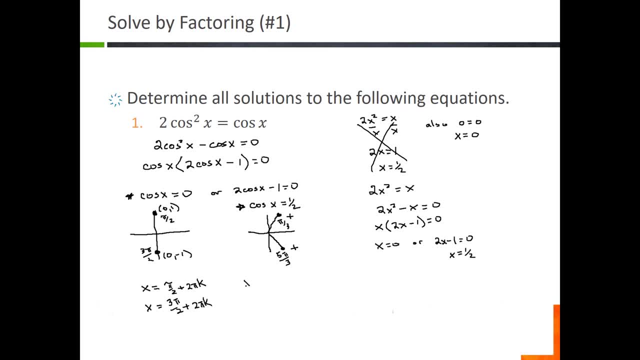 So if we write those out and expressing the infinitely many solutions we'll have x equals a pi over three plus a two pi k. And then we'll also get a five pi over three plus a two pi k. So all four of these answers together. Okay. So. Okay. 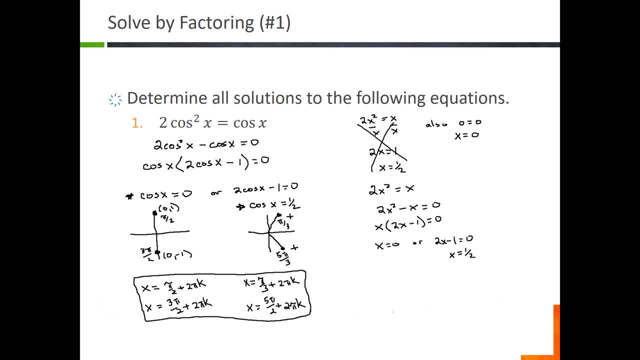 So if we wanted to write out the infinitely many solutions we'd have to list all four of those out. 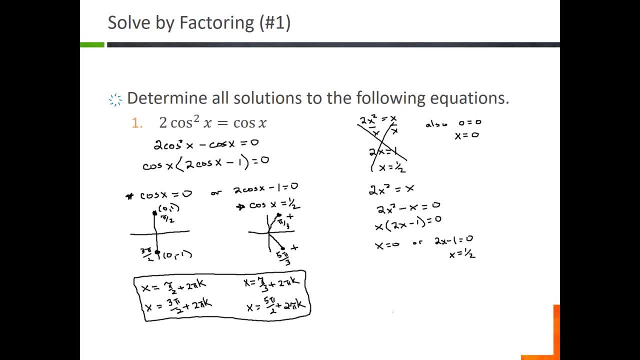 If you wanted just the answers between zero and two pi it's the pi over two, the three pi over two, the pi over three, and the five pi over three. 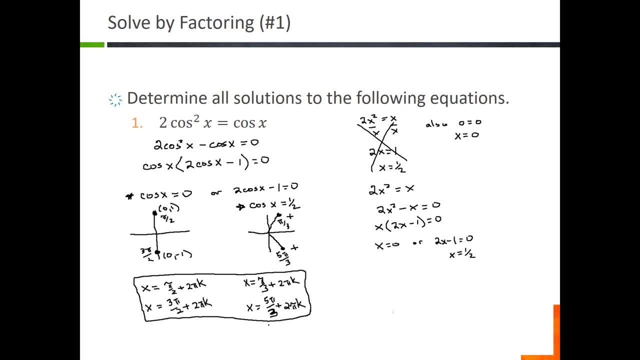 This should be a three here. Alright. 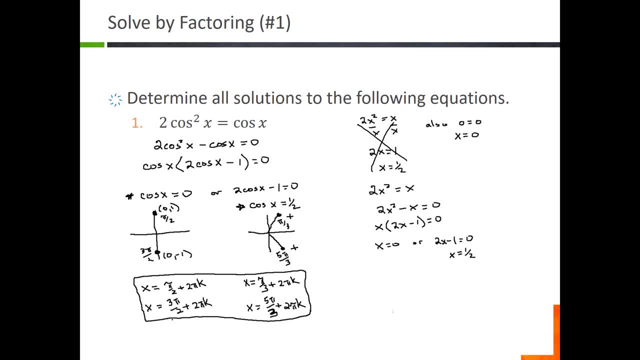 Now technically I'm not too worried about this. But in case you see it here. Uh. 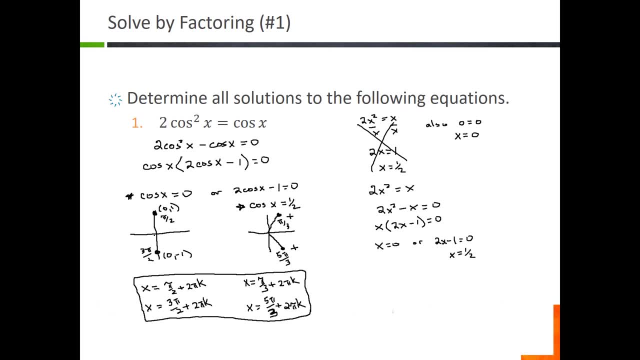 The pi over two and the three pi over two those are both a distance of pi apart. So from pi over two to three pi over two is a distance of plus a pi. And from three pi over two up to five pi over two is another distance of plus pi. So we could take these first two. And rewrite them as just pi over two plus pi k. Okay. 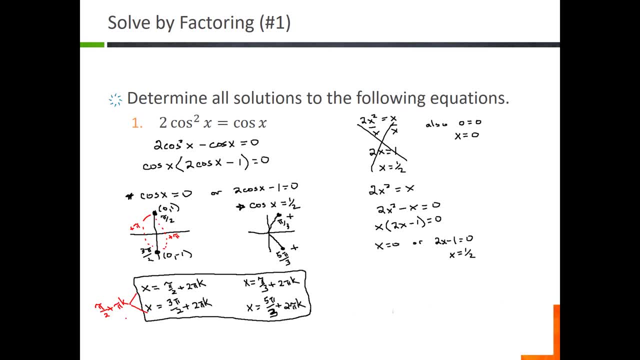 So I could merge those together into just a single expression. But I can't do that with the pi over three and the five pi over three. So whether you're either going to have all four answers, all four expressions as your answer. 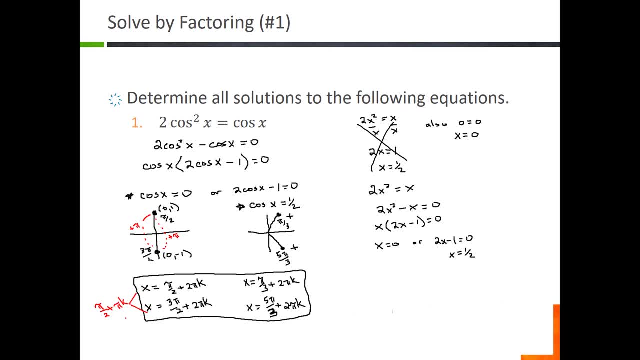 Or if you merge the two you'll have the three answers as your expression. The pi over two plus pi k. And then the pi over three plus two pi k. And then the five pi over three plus two pi k. Like it. It doesn't matter to me which way you do it. But just in case you have any questions. I'll be happy to answer them. 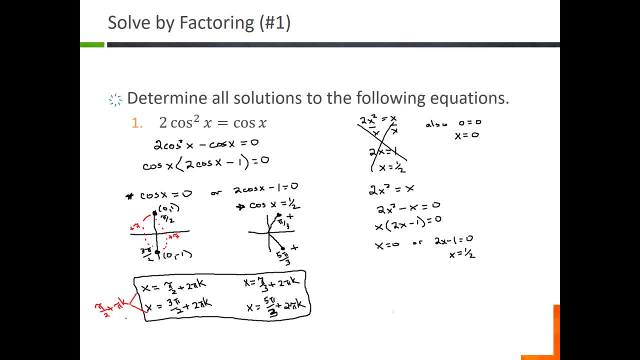 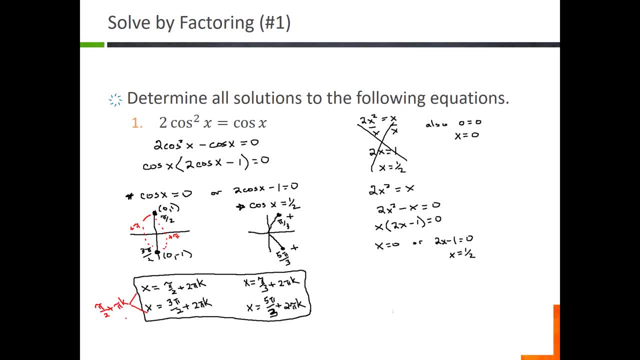 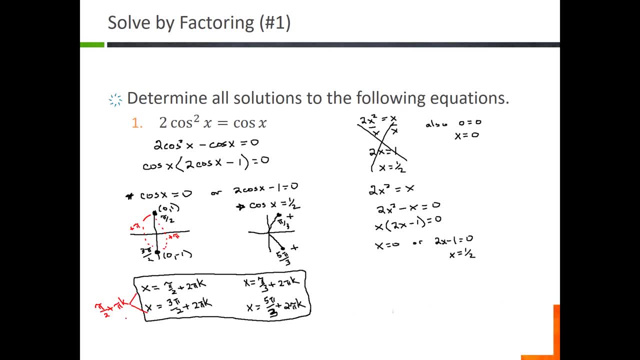 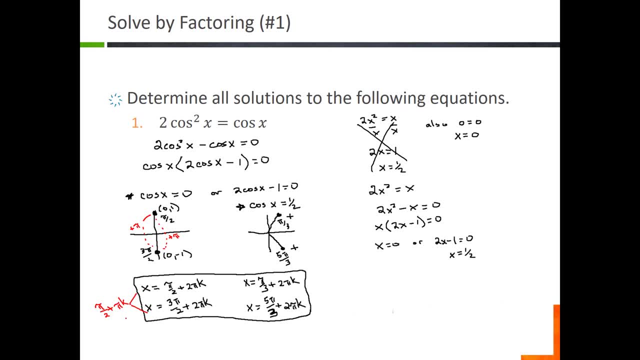 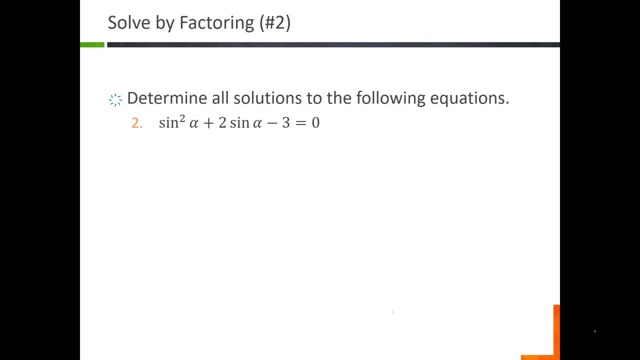 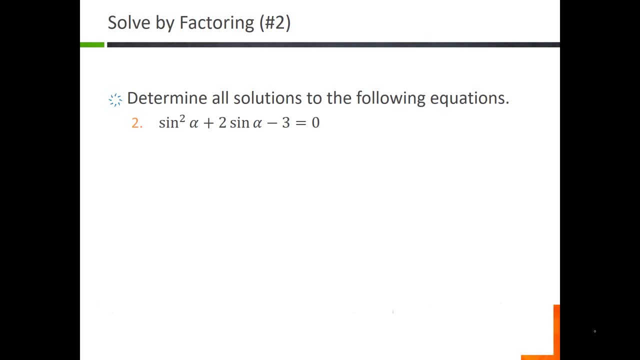 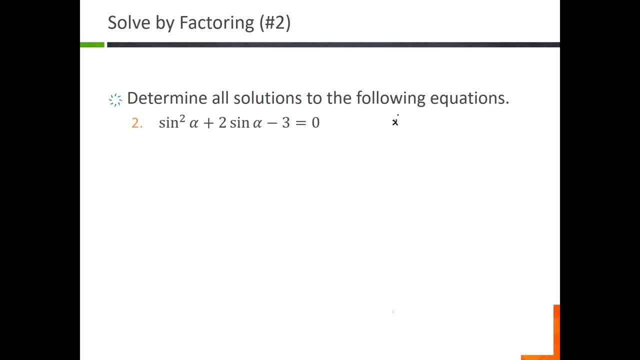 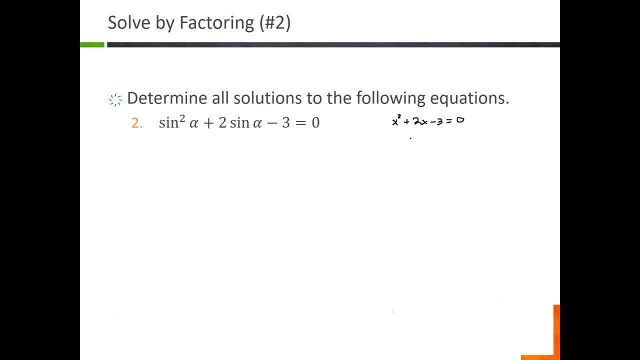 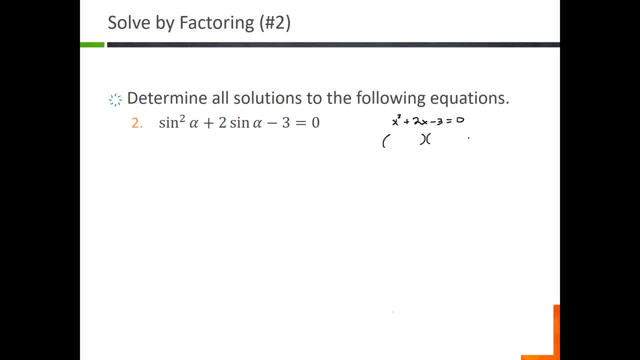 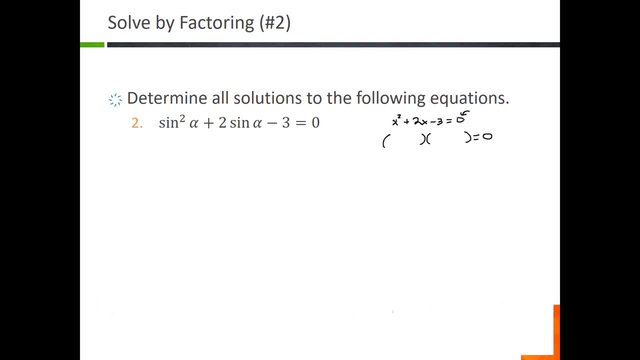 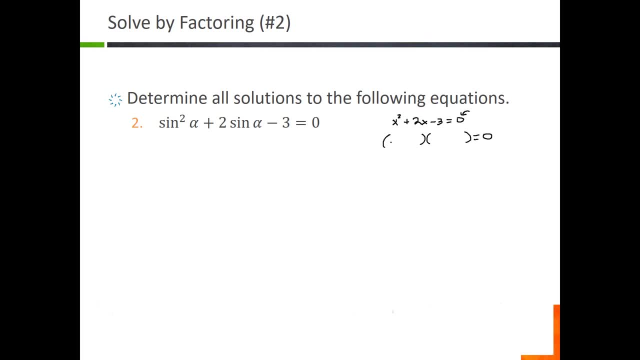 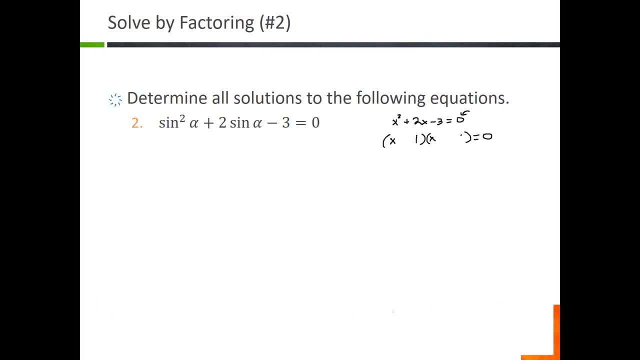 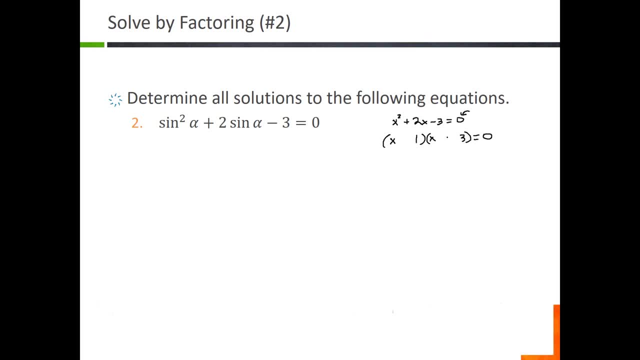 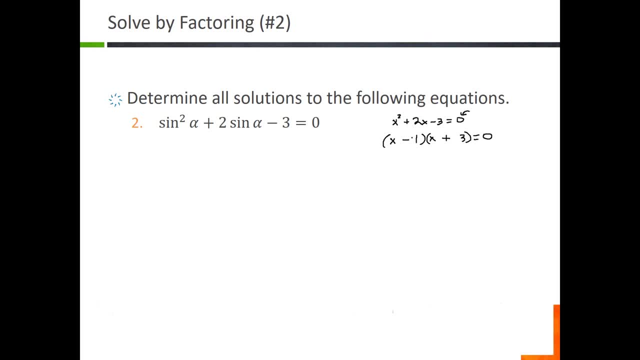 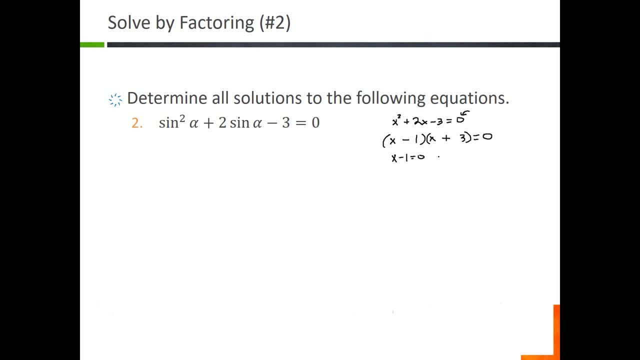 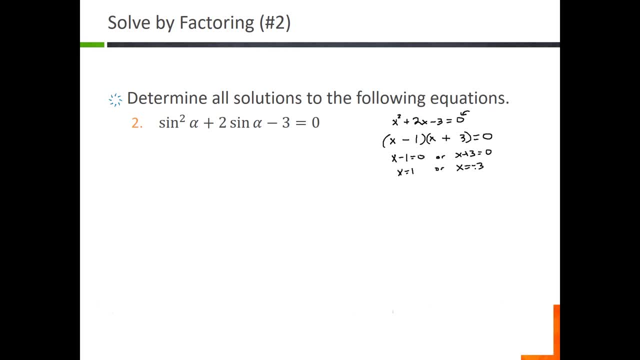 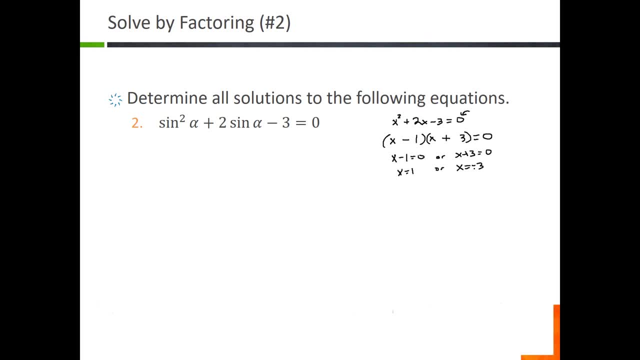 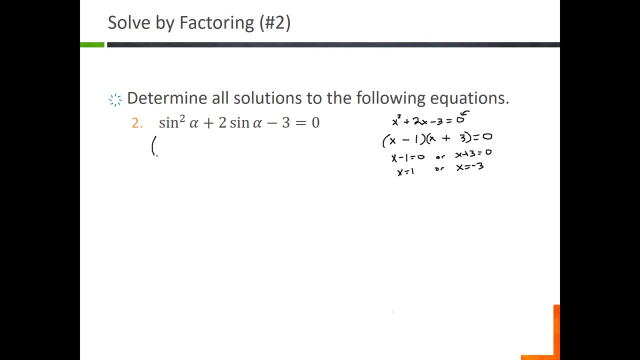 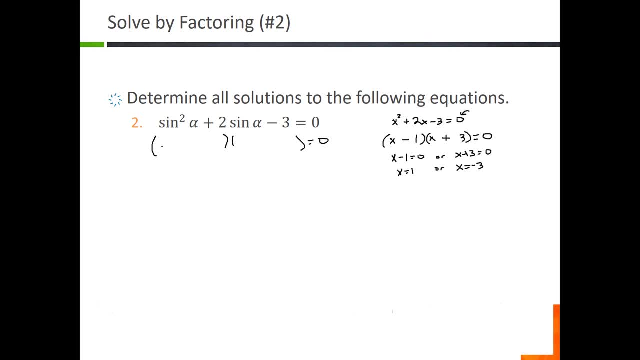 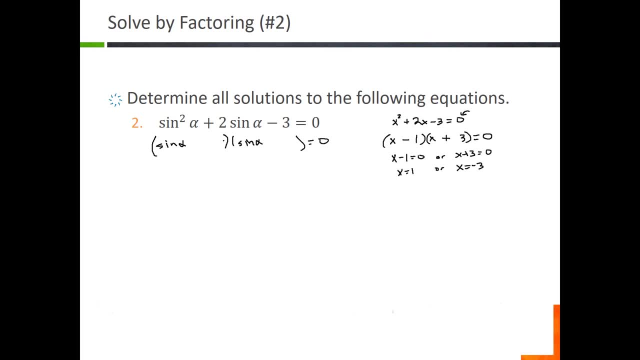 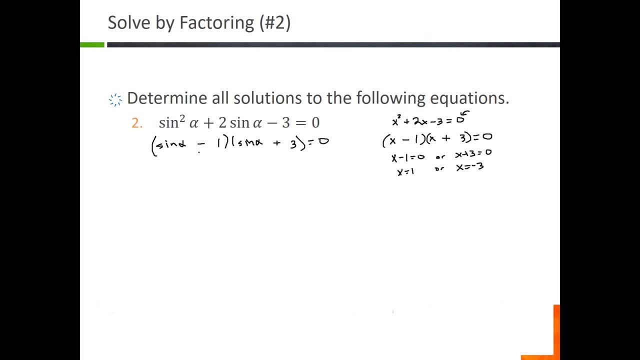 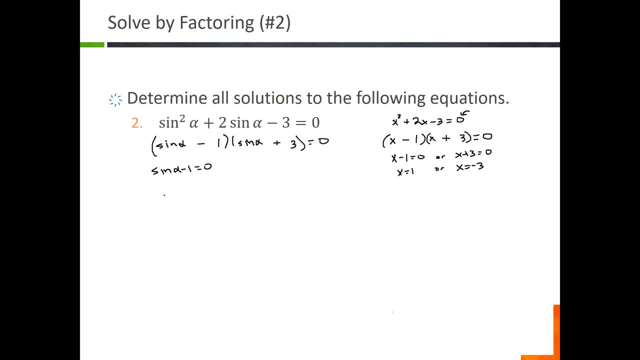 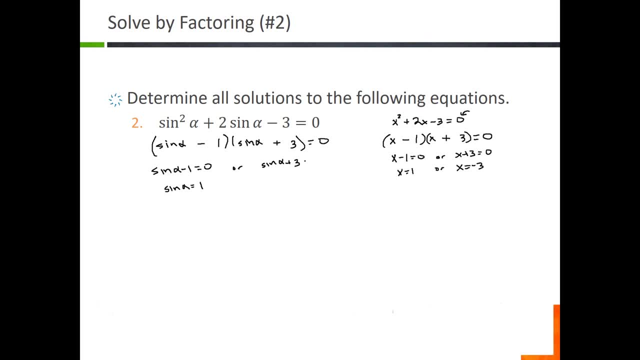 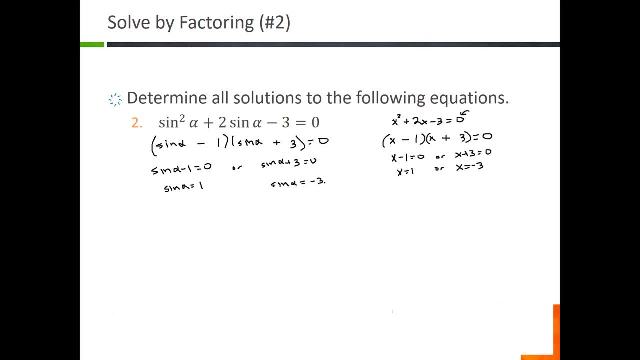 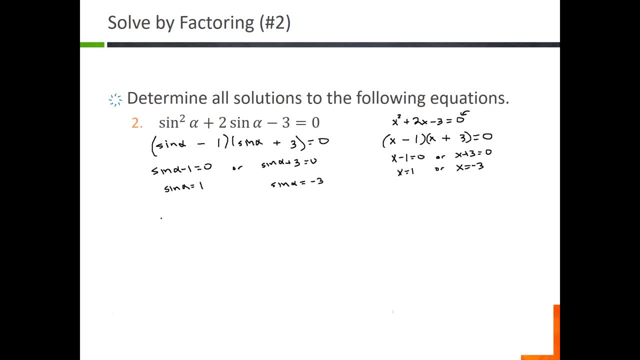 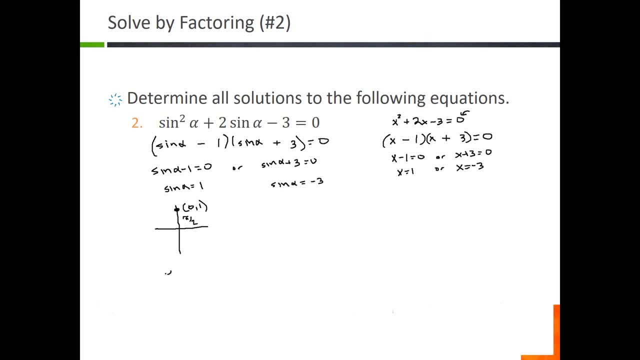 So that means right now we have theta is equal to pi over 2, and since we're wanting to find all solutions, we'll just put a plus 2 pi k on there. If I only wanted the solutions between 0 and 2 pi, I would just say pi over 2, and that would be it. 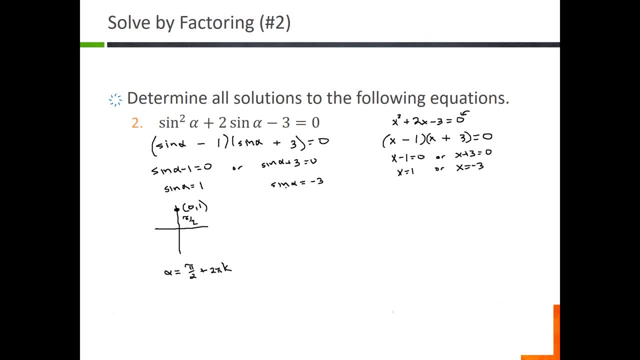 Alright, let's talk about our second equation over here. We have the sine of alpha is equal to a negative 3. So this is actually going to turn out really nice for us, we just got to think about it a little bit. 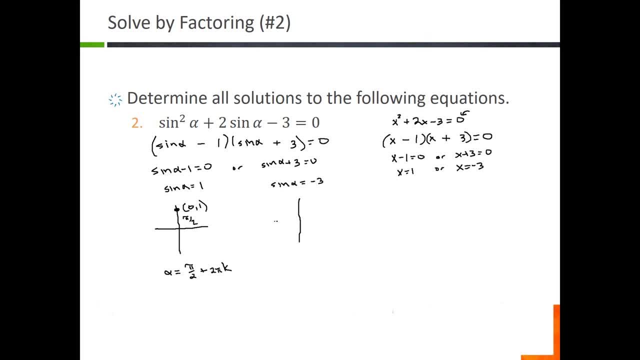 If you think about the unit circle, remember sine represents the y coordinate. What's the highest y coordinate we have? It's the point 0, 1. So the highest sine ever gets is 1. What's the lowest it ever gets? If you go to the bottom of the circle, it's the point 0, negative 1. 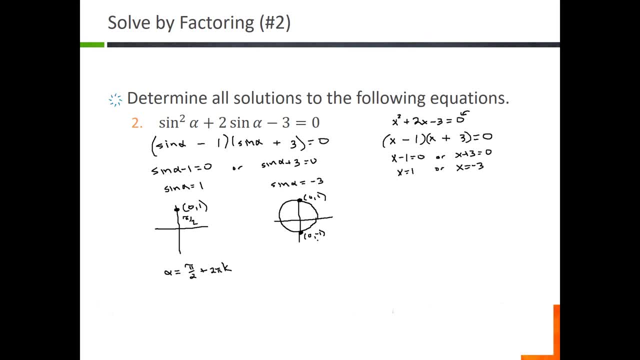 So the highest sine ever gets is 1, the lowest it ever gets is negative 1. If you go back to the trig graphs, the sine graphs that we saw a few weeks ago, the sine wave goes up and down and then back up to the origin, so it has that kind of shape. And it's range is from negative 1 to 1, remember? 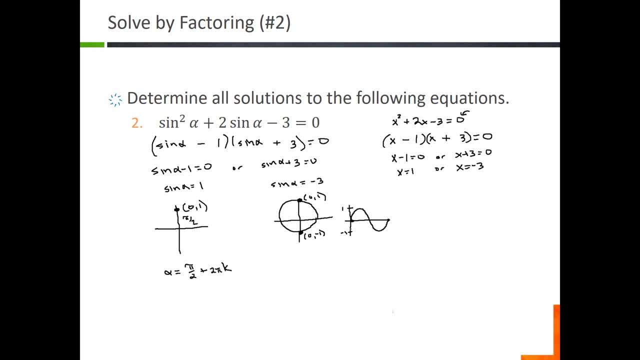 So it doesn't go both ways. It doesn't go below negative 1 and it doesn't go above a positive 1. 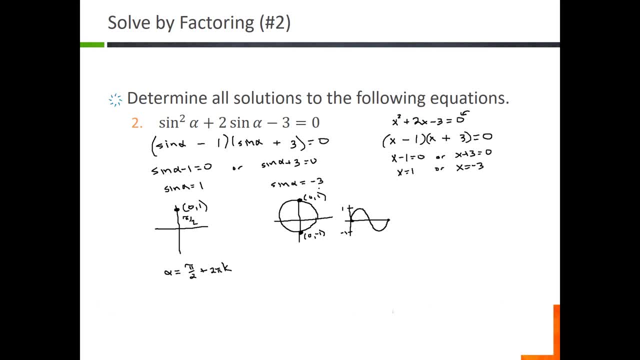 So how is it possible to get sine equal to a negative 3? Well, the answer is that it doesn't. So this particular part of the equation does not give me a solution, or you could say it does not exist. So there is no solution for this half of the equation. 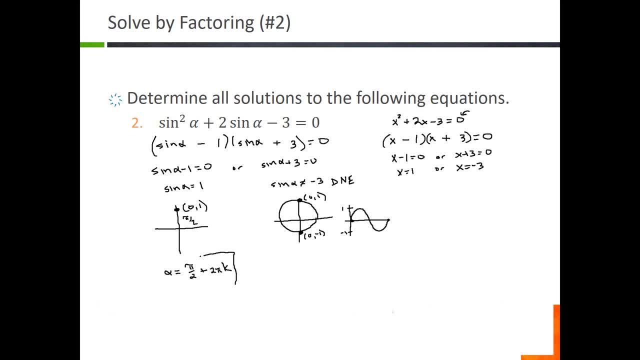 Which means the only solution I have to worry about, the only solution to my original equation, is my pi over 2 plus 2 pi k. Alright, last example. 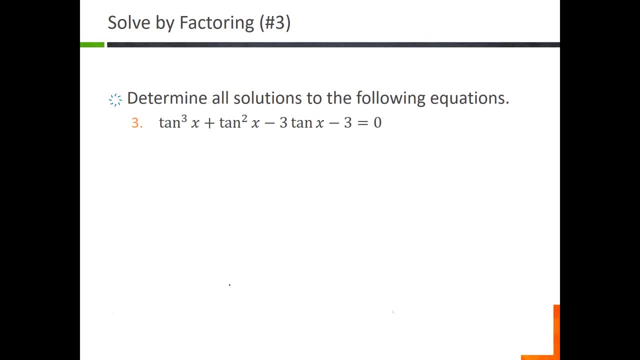 Again, dealing with factoring, just we're going to add a term onto this one. So we have the tangent cubed of x plus the tangent squared of x minus 3 tangent x minus 3 is equal to 0. Okay? 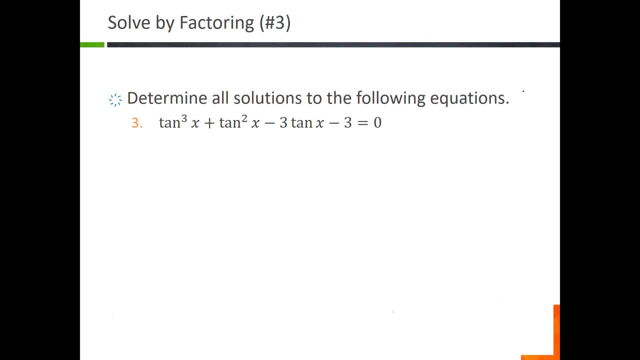 So let's try to do this again, just knock off all the tangents. Let's think of this as x to the third plus x squared minus 3x minus 3 equals 0. And the x's in my algebraic equation represent tangent x. 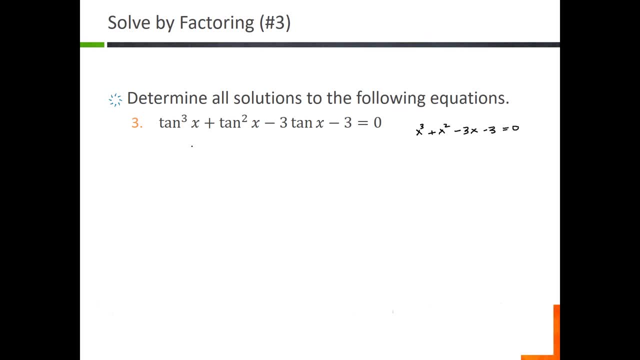 Where tangent x over here is a different x. But anyway, we're just playing around here. 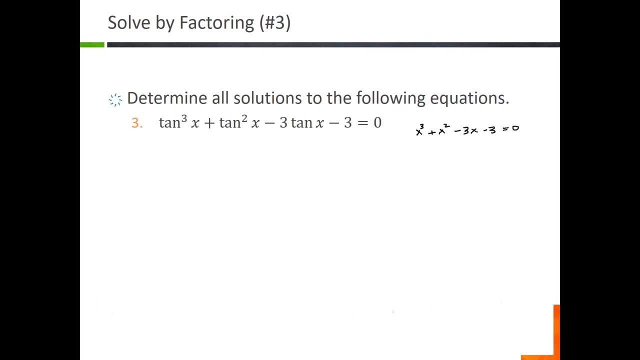 So how do we factor x cubed plus x squared minus 3x minus 3? Some of you may remember this. But we're going to use a process called factoring by grouping. Okay? So we're going to pair up our terms. There's four terms, we're going to pair them up. So what can I pull out? What do I have common between x to the third and an x squared? Well, I can pull an x squared out of both of those. 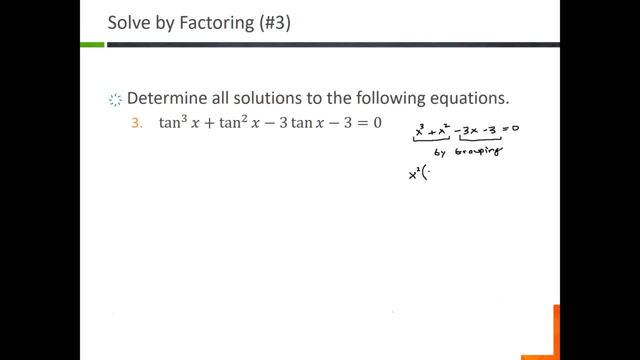 And if I pull an x squared out of those, we're going to be left with an x plus a 1. All right? 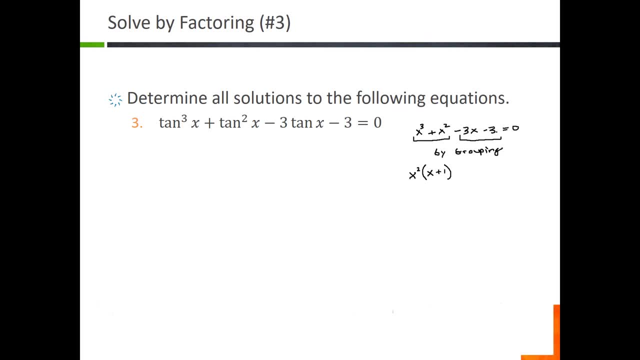 And what can I pull out of a negative 3x minus 3? They both have a 3. And they actually both have a minus or a negative. So let's pull out a minus 3. So if we pull out that minus 3, we're left with an x plus a 1 again. Okay? And so now we have two groups. 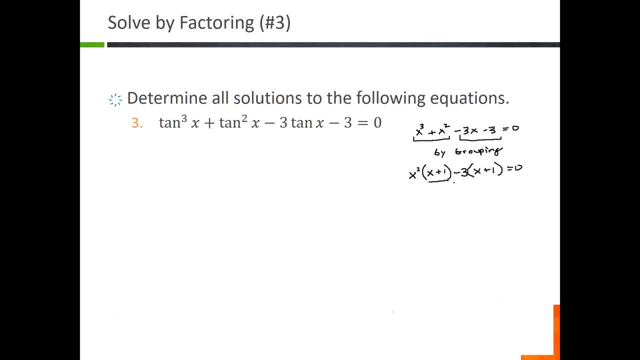 We have the x squared times x plus 1. And then we have the minus 3 times another x. Well, those x plus 1s, those are common factors. So we can pull those out front just like we did before. So we're going to pull out an x plus 1. And we're going to be left with an x squared minus 3. And that will all be equal to 0. 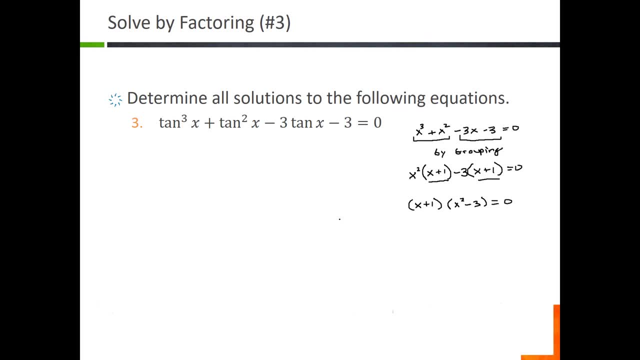 And then we can solve the equation from there. So that's going to give us x plus 1. 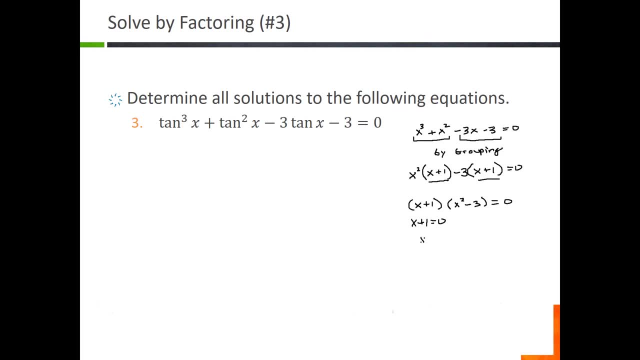 x plus 1 is equal to 0. Which means x is equal to a negative 1. And then we're going to have x squared minus 3 is equal to 0. Which means x squared is equal to a positive 3. Which means x is equal to a plus or minus square root of 3. Okay? 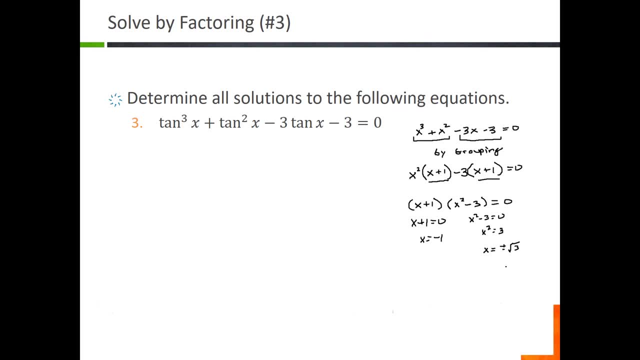 So we're going to do the same thing using the tangents that we just did using just the x's. So we're going to follow the same algebraic process. Just using graphs. 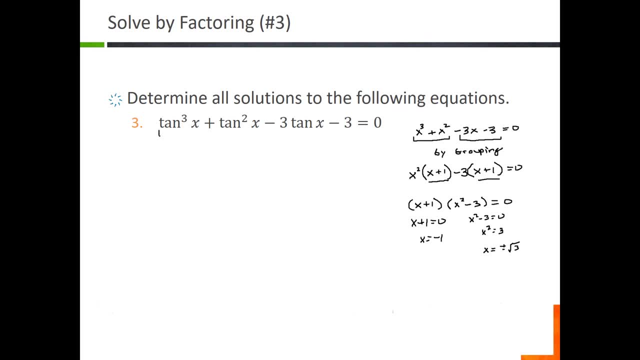 Using tangents. So we're going to group the tangent cubed and the tangent squared. And then we're going to group the negative 3x minus the 3. So we're going to pull out a tangent squared x. Which leaves a tangent x plus 1. And then we're going to pull out the minus 3. Which is going to leave another tangent x plus 1. Still equal to 0. Both of these terms now have a tangent x plus 1. 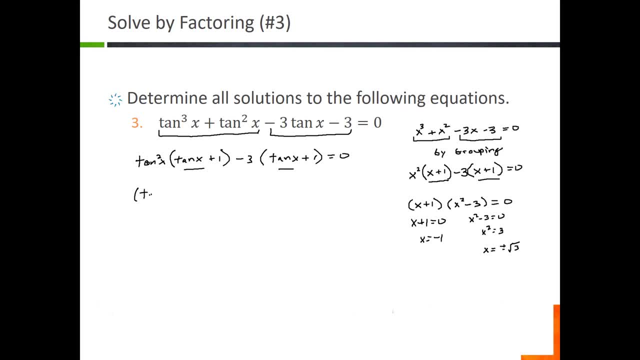 So we're going to pull that out front. We have a tangent x plus 1 times a tangent squared x minus 3. Still all equal to 0. 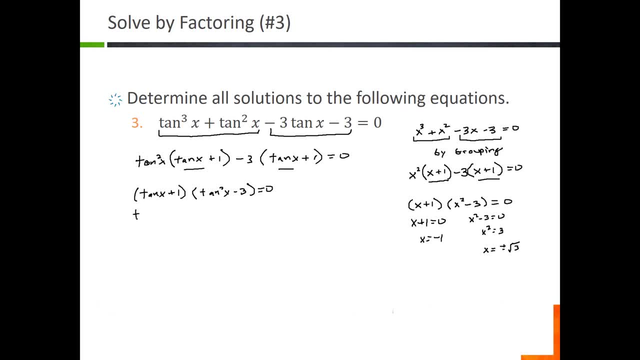 And then we're going to split those apart. So we have the tangent of x plus 1 is equal to 0. 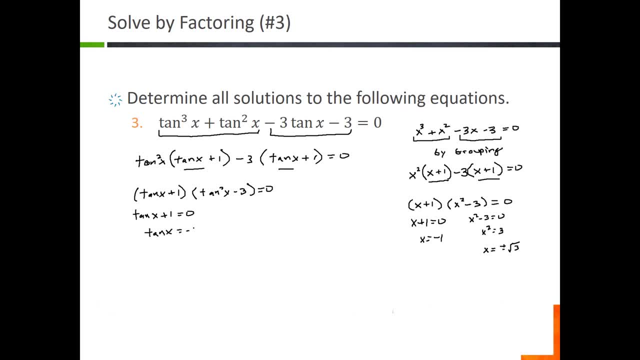 Which means the tangent of x is equal to a negative 1. 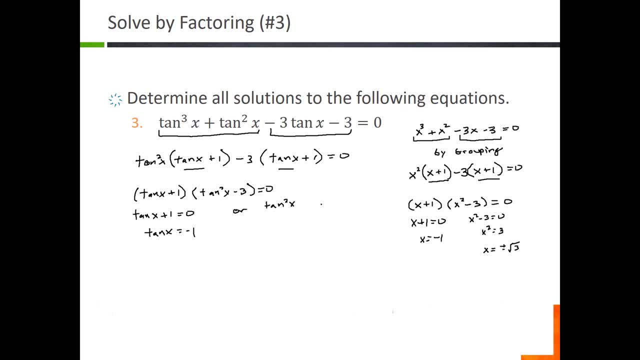 Or we have the tangent squared x minus 3. Minus 3 is equal to 0. 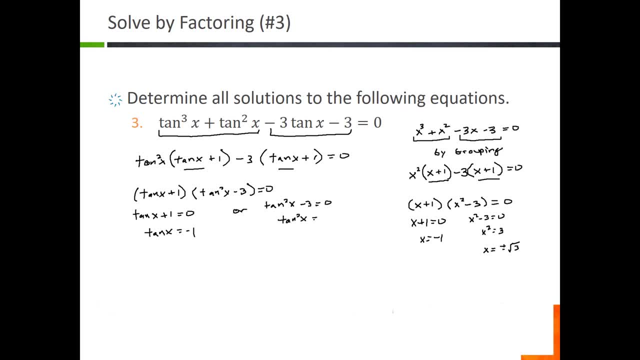 Which means the tangent squared x is equal to a positive 3. 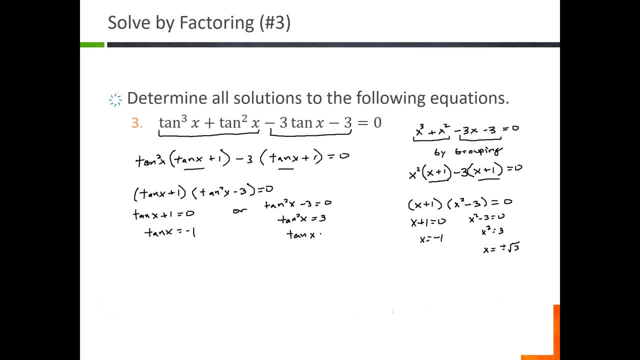 Which means the tangent of x could equal a positive or a negative root 3. And let's split that apart now. 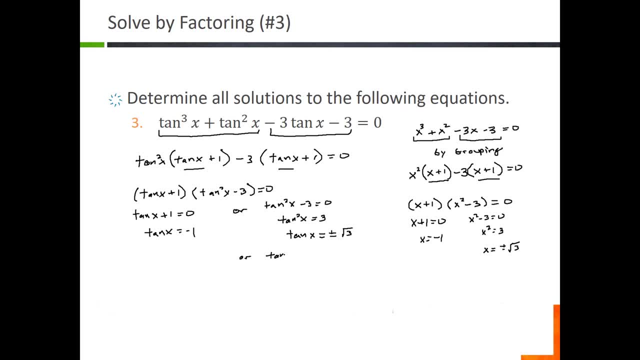 So that means we have or the tangent of x is equal to a positive root 3. Or the tangent of x is equal to a negative root 3. 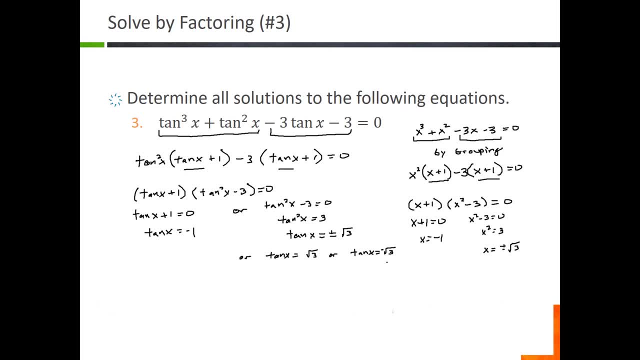 So in this example we actually have three equations that we need to check their solution. And then we want to find and express all of our answers. So let's look at, let's go back to tangent of x equals negative 1. So we know tangent is positive in the first and the third quadrant. And it's negative in the second and the fourth. 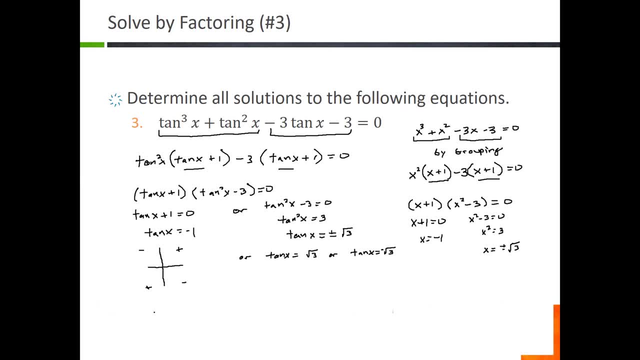 So we need an angle in the second and the fourth quadrant. And we know that since tangent is equal to 1 it's equal to y over x. That's equal to our, it's going to be at our 45 degree angle or our pi over 4 angles. So if we look at pi over 4 in the second quadrant that will be 3 pi over 4. And in the fourth quadrant it's going to be 7 pi over 4. So we have two angles. Alright. 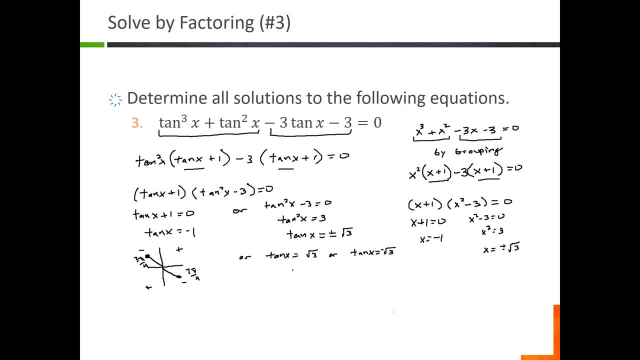 If we look at the tangent of x equals square root 3. Again let's draw our unit circle here. 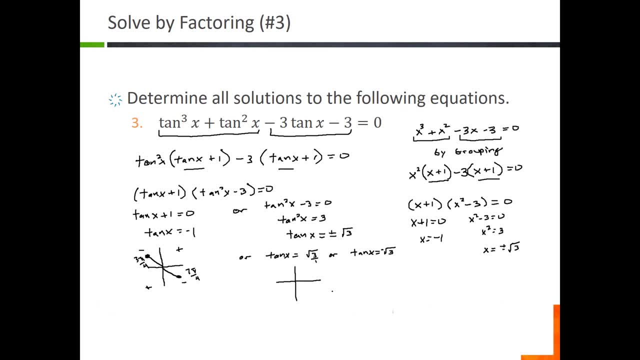 Think of square root of 3 as square root of 3 over 1. 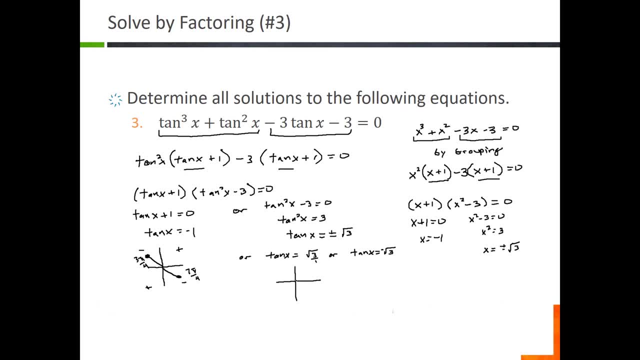 It's positive so that's going to be somewhere in the first quadrant. But it's also positive in the fourth, second, third quadrant sorry. So first and fourth. 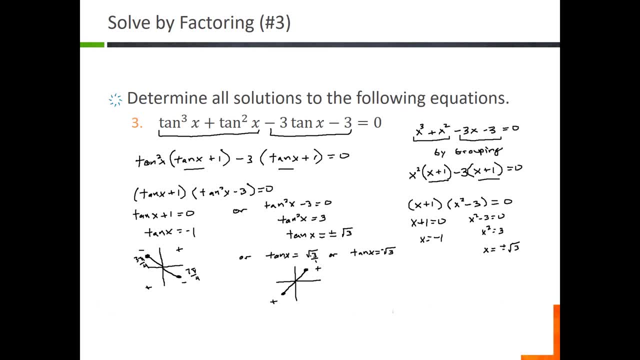 And remember sine, tangent is sine over cosine. So when is sine root 3 over 2. Again this is kind of the way I do it. What is it? 3 over 2 and 1 over 2. 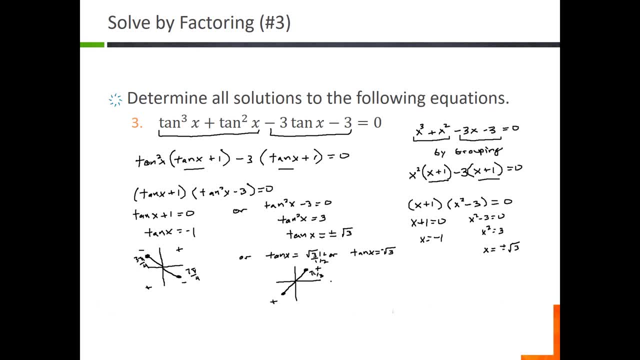 That would be at the pi over 3 angle. So we have a pi over 3 in the first quadrant. 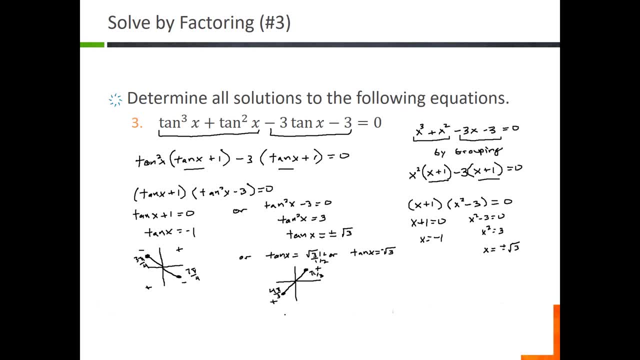 And then we're going to have a 4 pi over 3 in the third quadrant. So we have two more. 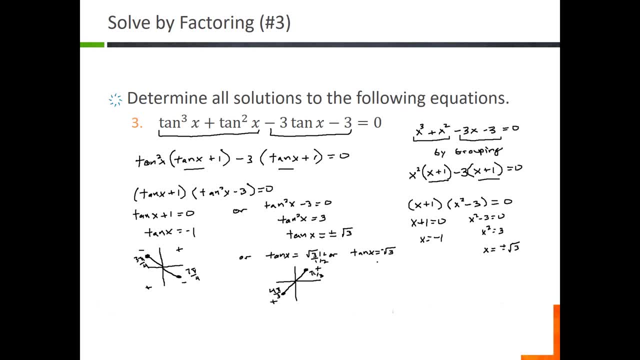 And then the last part here is tangent of x equals a negative 3. 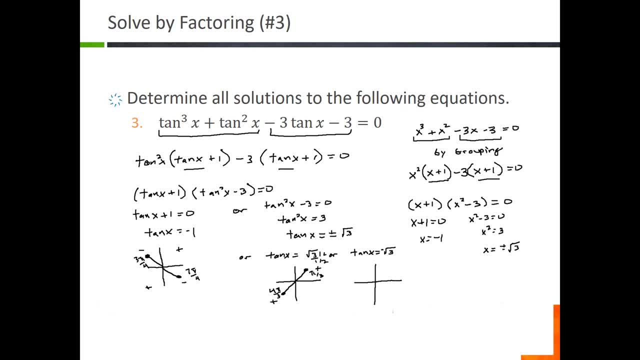 Well same basic thing we just looked at. But it's negative which tangent is negative in the second and fourth quadrants. But it's still basically just a root 3 over 1. 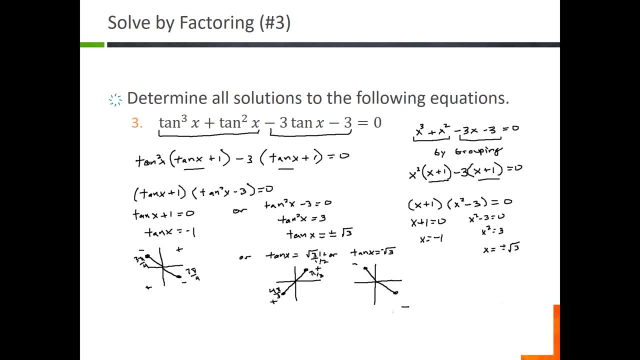 And so that's going to put us at pi over 3 angles in the second and fourth quadrants. 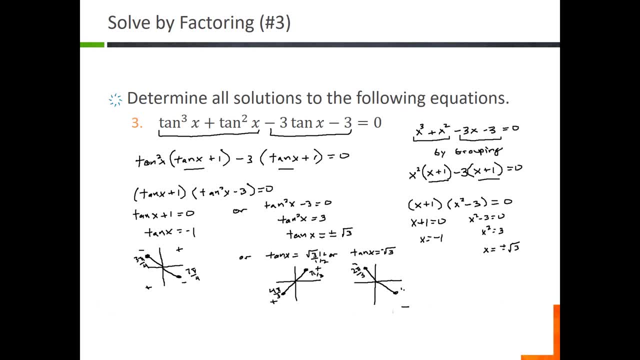 So 2 pi over 3 and 5 pi over 3. So between 0 and 2 pi we have 6 answers. 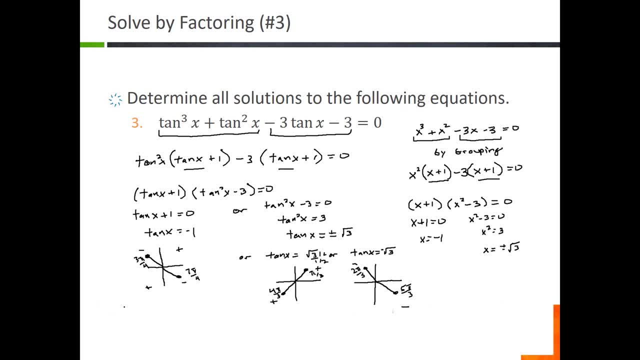 Okay so let me just list all 6 of those out. So between 0 and 2 pi. 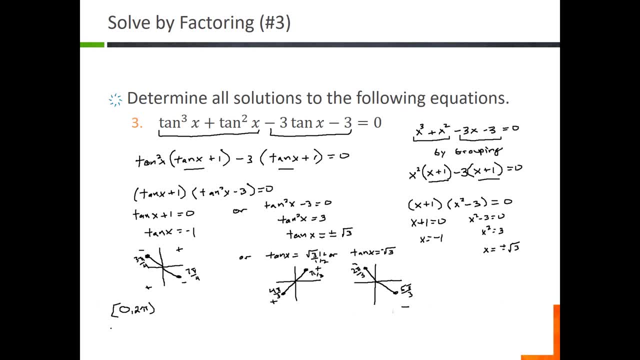 We have x could equal. Let's try and list them off in increasing order. So we could have pi over 3. We could have 2 pi over 3. We could have 3 pi over 4. 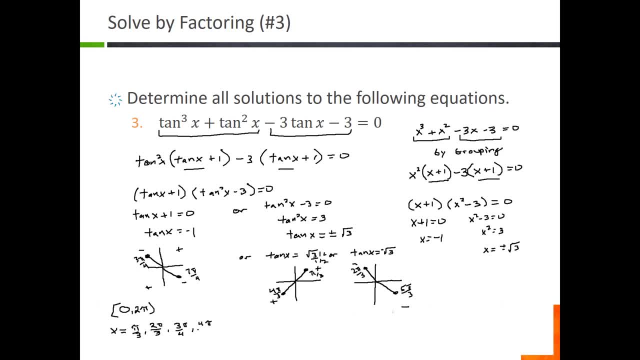 We could have 4 pi over 3. And then we could have 5 pi over 3. And then lastly we would have 7 pi over 4. 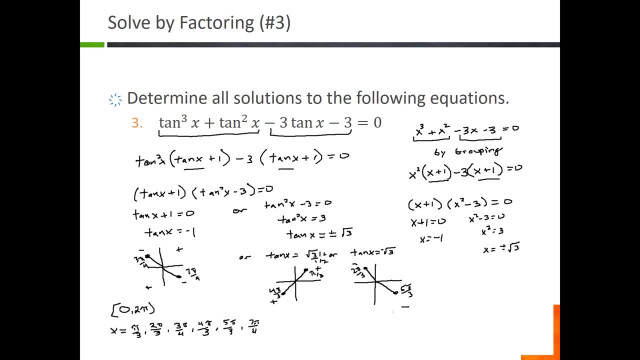 Now if you don't list them out in order that's fine. But so we have 6 possible answers here. Okay and if you're just trying to list the answers from 0 to 2 pi you have to list all 6. 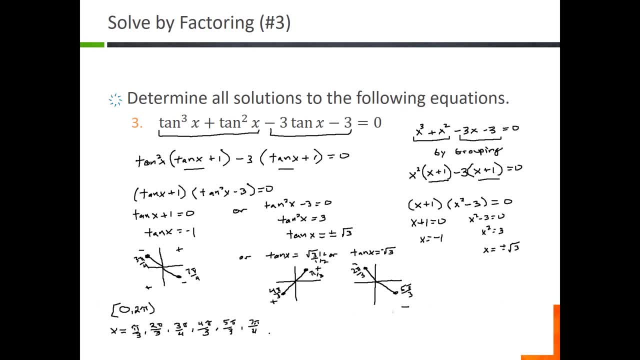 Okay but we just want to list the infinitely many solutions. So let's remember how we do infinitely many solutions with tangent. Okay remember the nice thing with tangent. 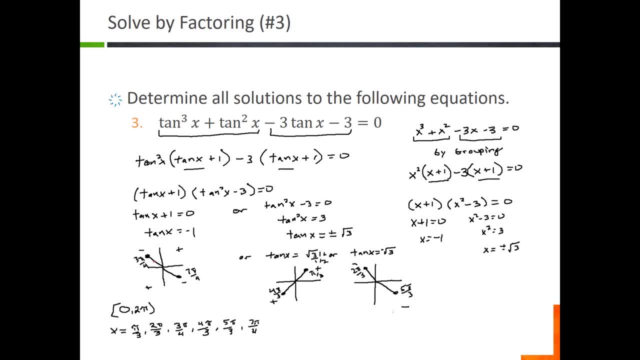 Tangent has a period of pi. So that means going from our first pair of solutions. 3 pi over 4 and 7 pi over 4. From 3 to 7 pi over 4 is a distance of pi. Where you're adding pi. And then coming around back to the starting point is another addition of pi. So we don't need to list both of these solutions. So we could just talk about. X equals we only have to list that first one. 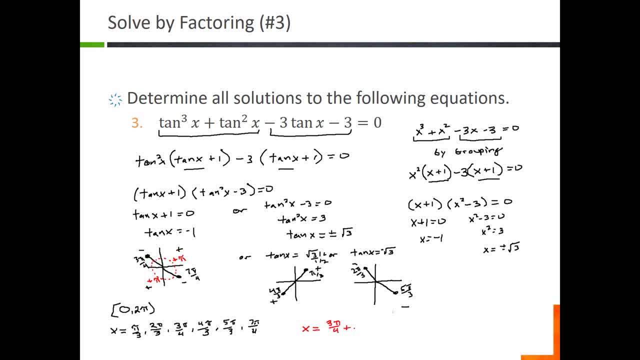 So 3 pi over 4 plus and we're going to do plus pi k. That's the first one.